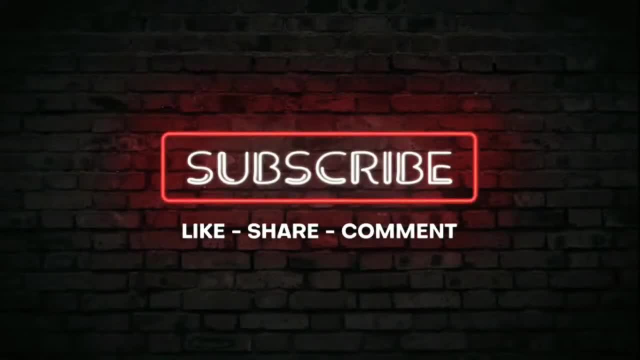 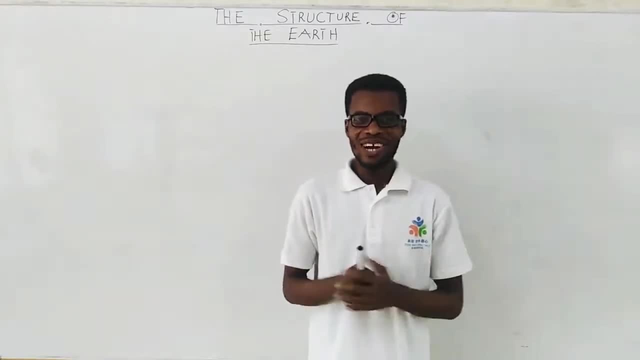 Hi, dear learners, Once again, you are welcome to GCSE Tutorials On this platform. as you already know, we teach you how to learn social studies, study the subject in a way that you can perform excellently in class and, at the same time, when you go out there, you become. 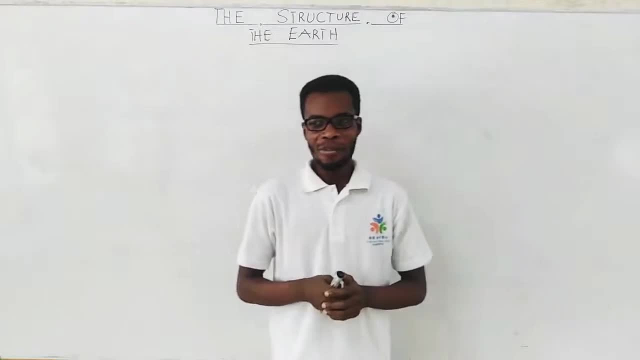 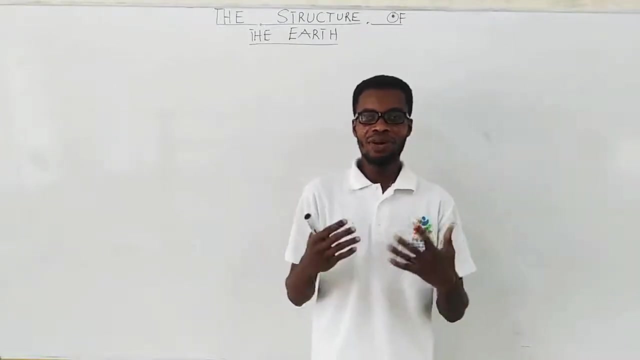 the responsible citizen that you wish you could be. We have treated a lot of topics on this platform. In our last lesson, we spoke about the revolution of the earth. This time round, I'm bringing you something talking about. we are moving away from space, getting 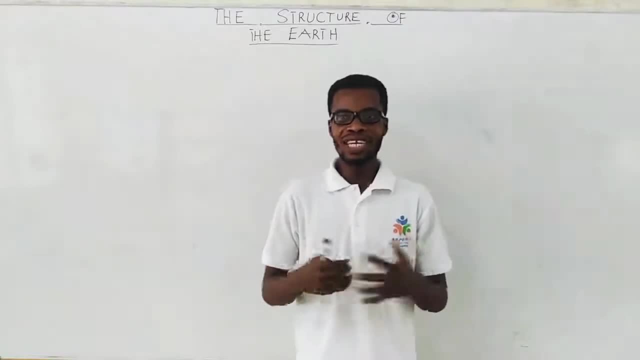 down on the earth to see what we have here on earth, and that is the structure of the earth. So by the end of this lesson, I expect you to know that various topics are being discussed. today We are going to talk about the various layers of the earth as a part. 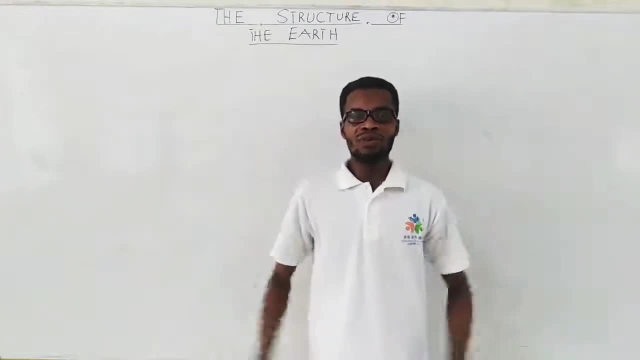 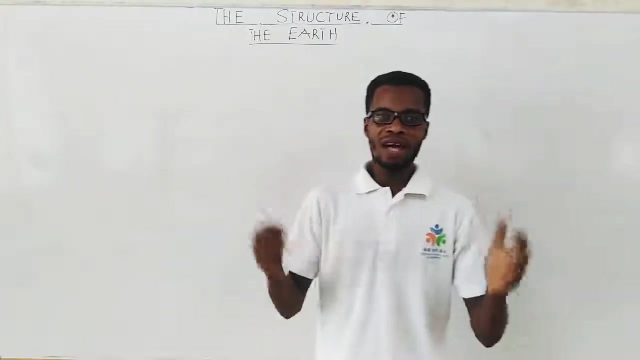 where we live or where we have a lot of human activities taking place. It's so interesting for you to know that there are layers or other structures under the path or the surface where we live, and we are going to delve into that. So our topic for today is the structure of 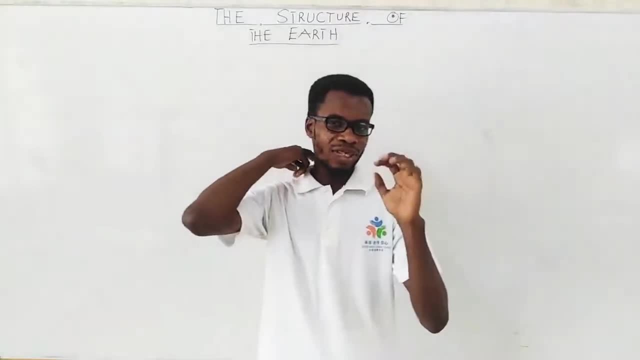 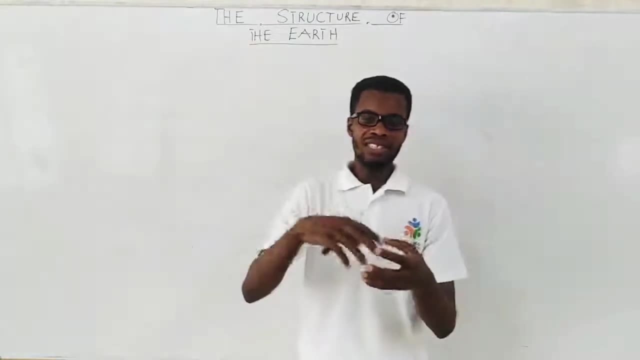 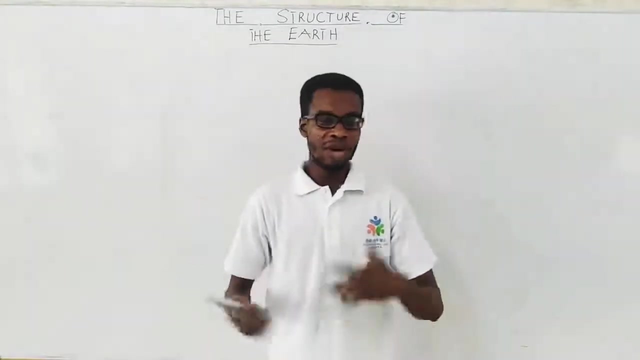 the earth. Now, when you pick an onion, you pick an onion, you realize that the onion is not in layers, So you pick outer shells, the outer, outer ones, and then you get to the innermost part When you pick other fruits, like coconut and mango, together with orange. 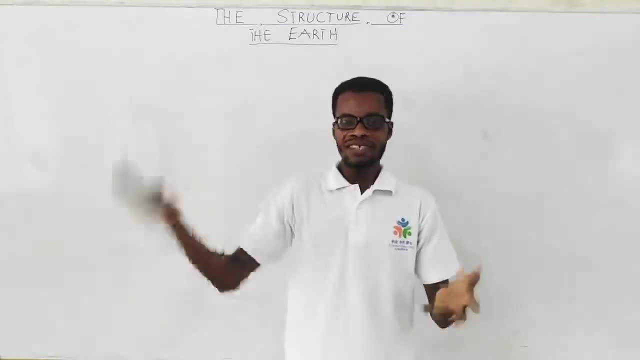 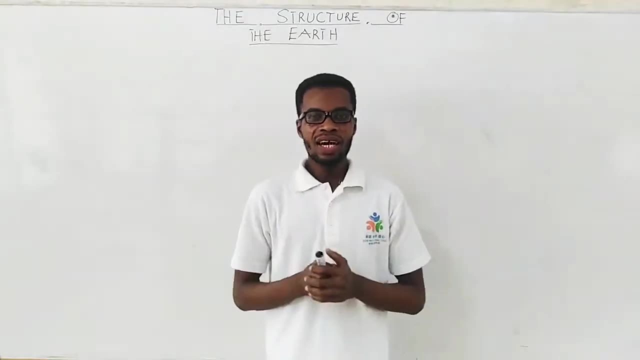 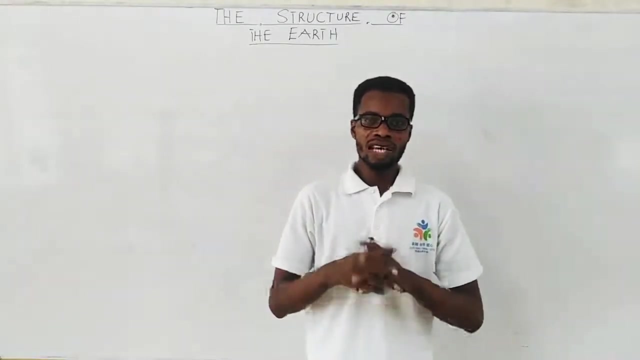 you find the same thing where you have to take off some layers, the outer one, before you get to the inner part or the innermost part. We have to look at the earth and view it in that same structure. The study of logs, that's timber- you realize that it has a cross-section and we have the 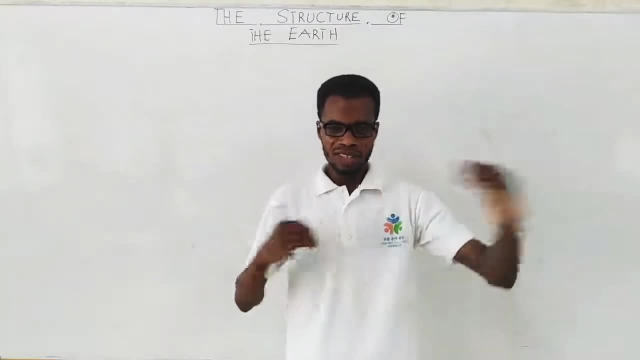 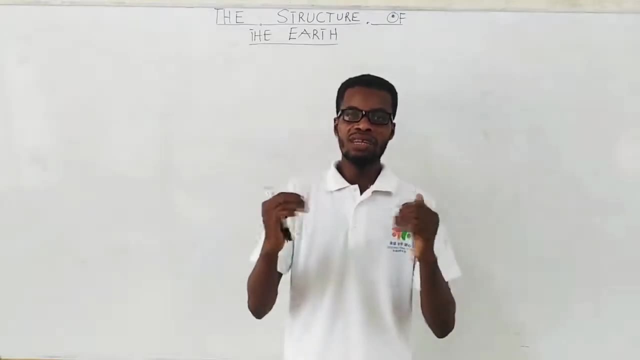 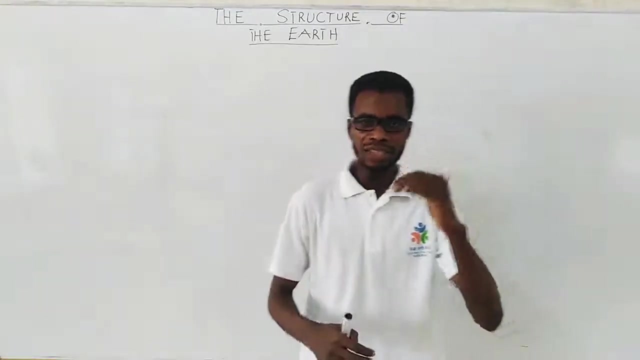 innermost part to the outer part of the log or the timber. Now the earth has that same structure, but we'll look at the various labels or names because the structure is different in terms of their qualities or what we can find in those layers. So we get to do that. 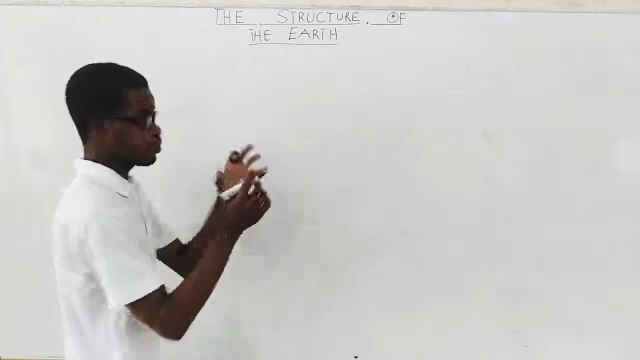 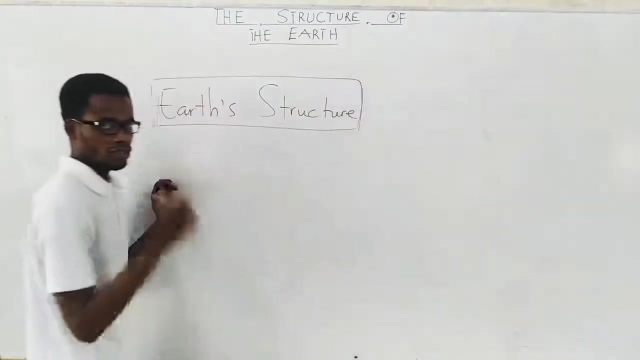 So when we pick. So if I want to use my spider gun to demonstrate that, if we have the earth's structure, we have what we call the core. From the core, then the mantle, Then from the mantle we have. 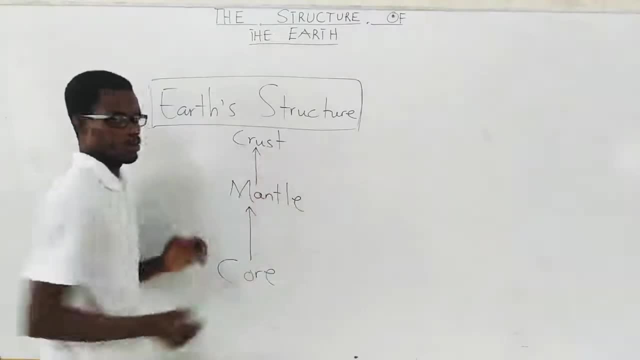 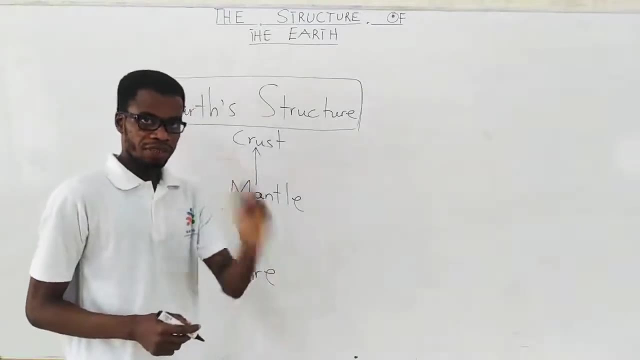 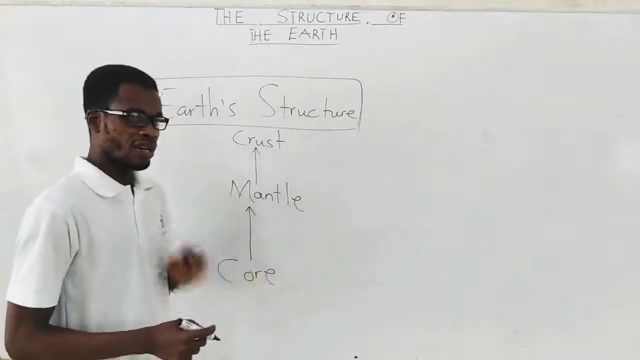 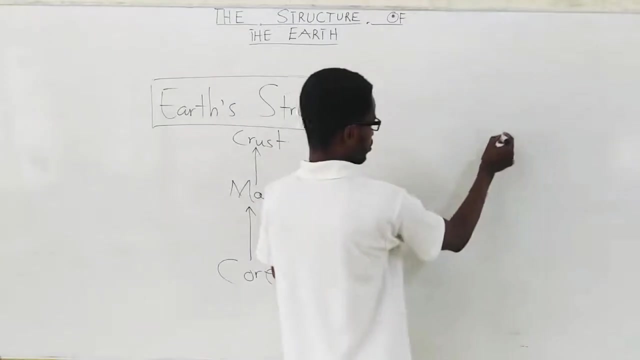 the crust. We get to the crust. We get to the crust. So three major layers. The earth's structure is divided into three major layers: Core, mantle, crust. So these are the three major layers. We'll take them one by one and we'll see how they look like So diagrammatically. 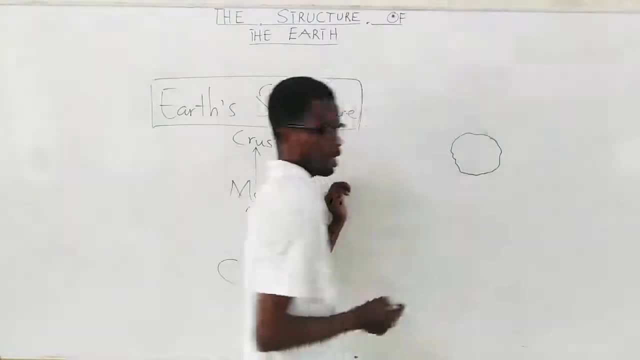 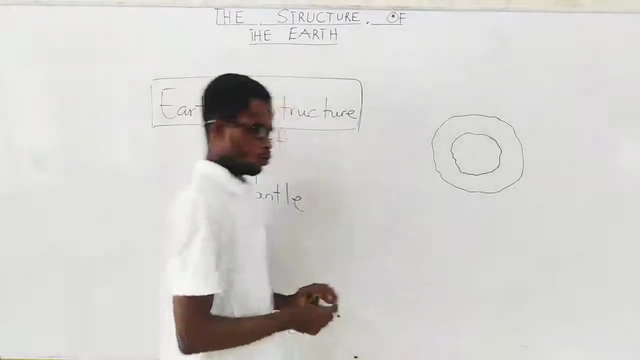 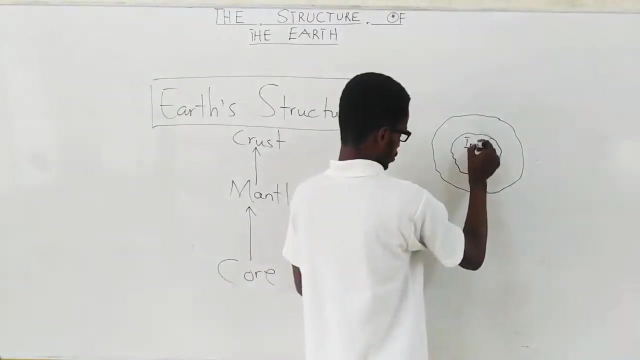 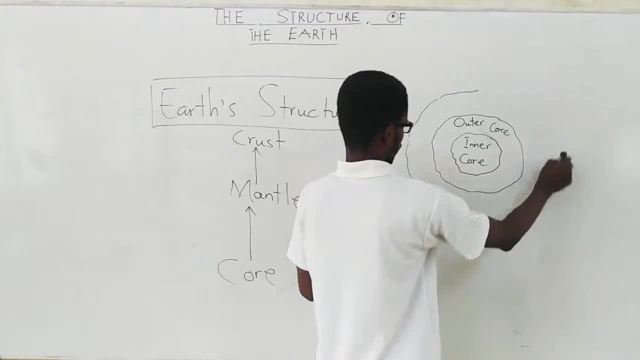 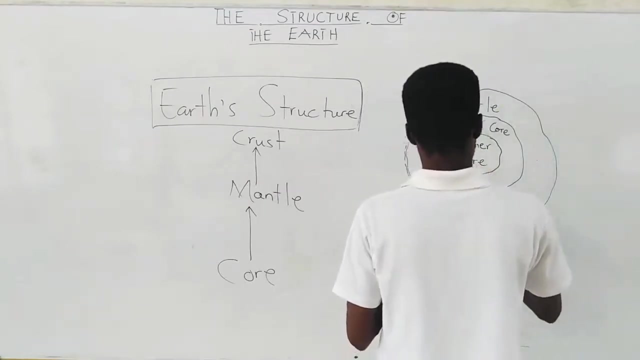 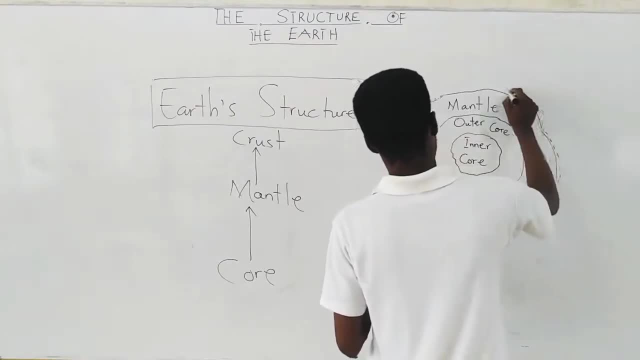 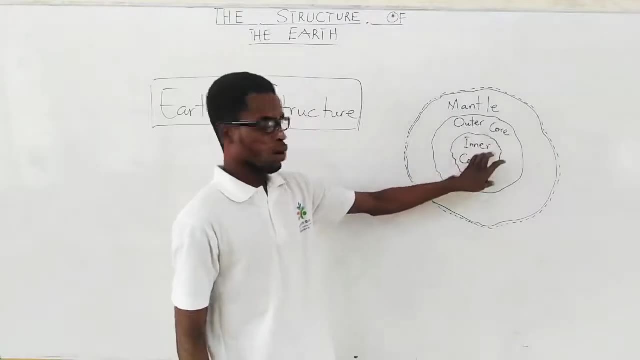 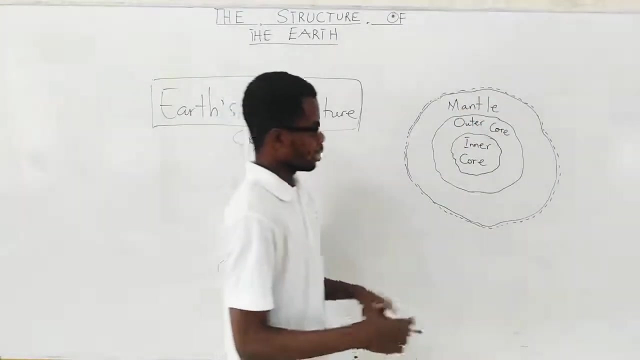 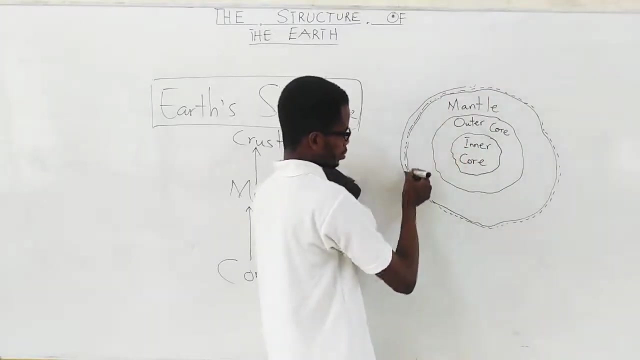 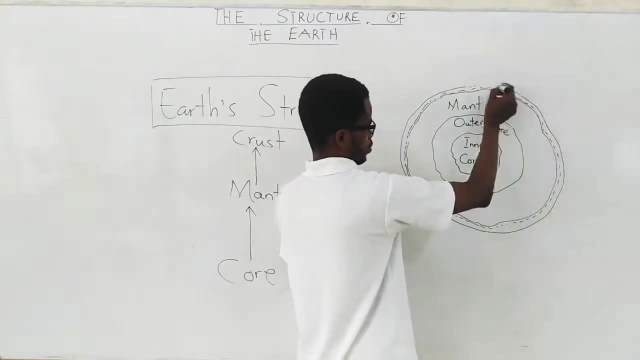 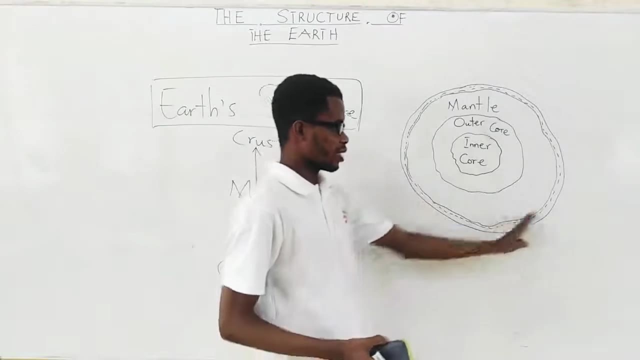 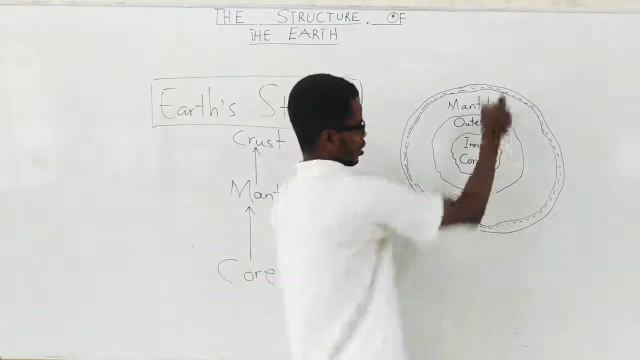 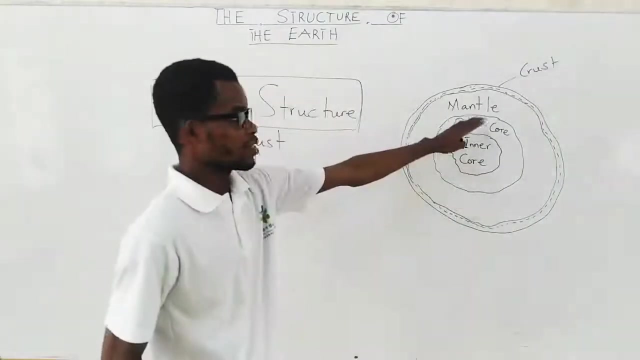 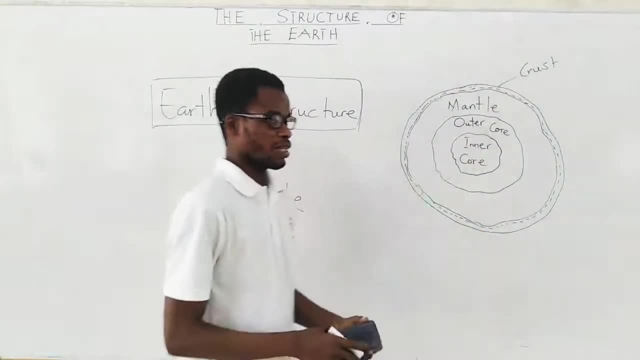 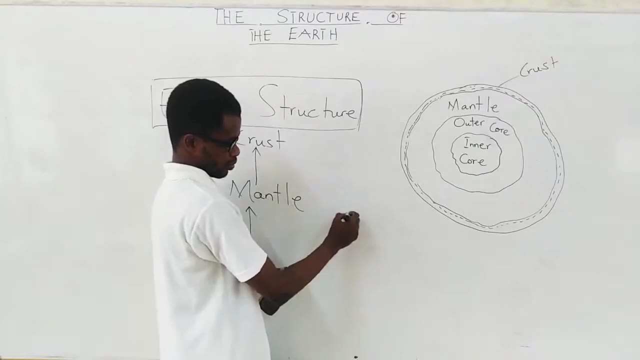 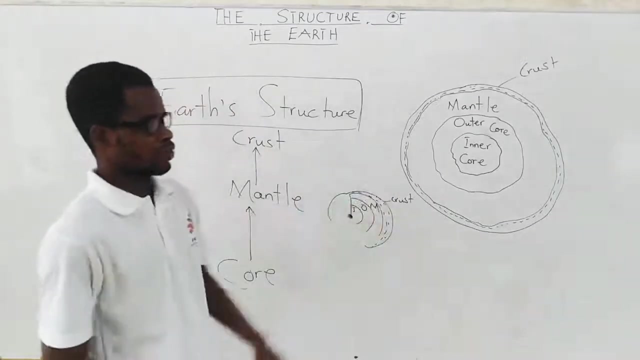 we find ourselves, the part where we find ourselves somebody to, we can decide to draw it locating the center of the earth, then maybe create the globe. so first inner core, outer core, mantle, and then that layer, the water, and then the crust. this can be another way of drawing it, but the circular cross section actually. 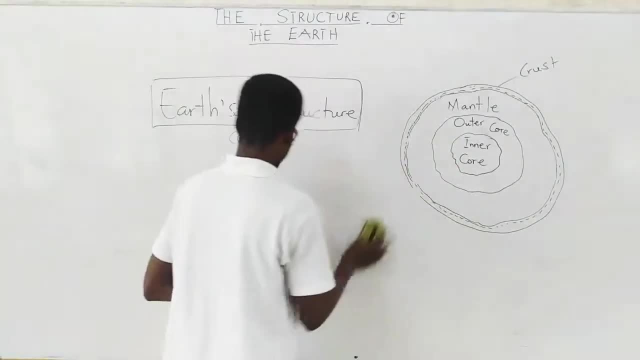 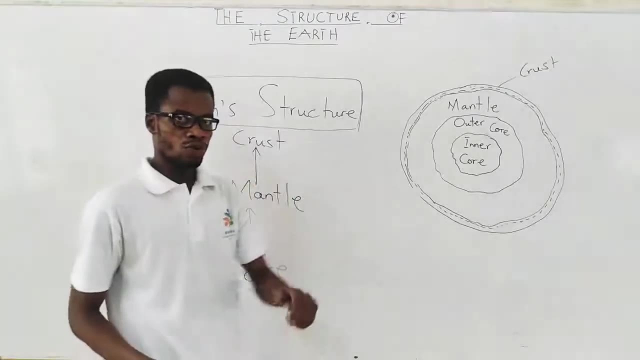 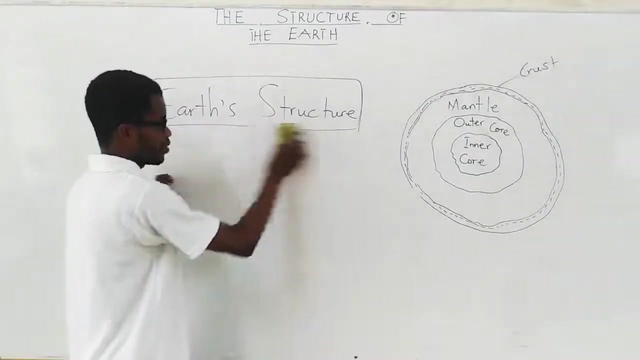 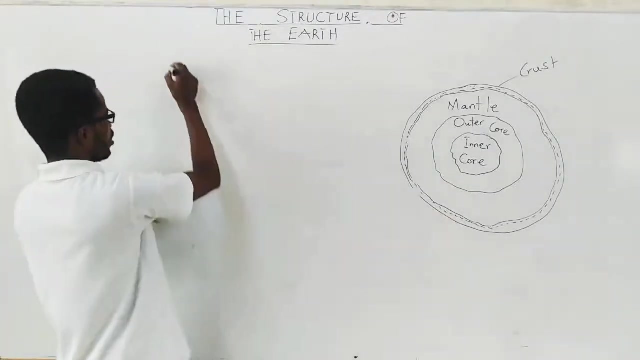 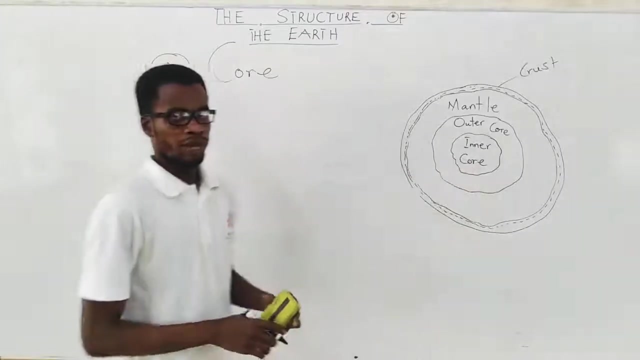 helps us to know what we are talking about. so three major layers, but the core is divided into two, so we take them one by one and see what we can find in these areas. so we begin with the inner part. let me just stay the core. the core is two parts, so the core is broken down. 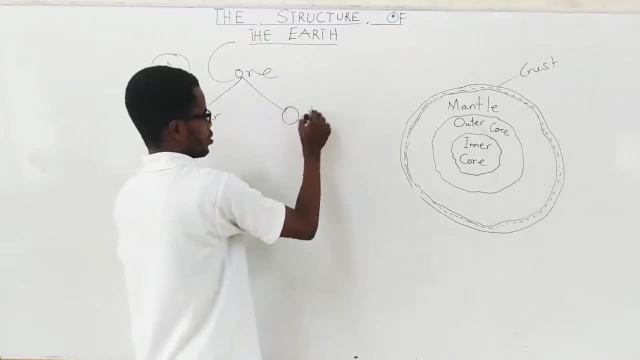 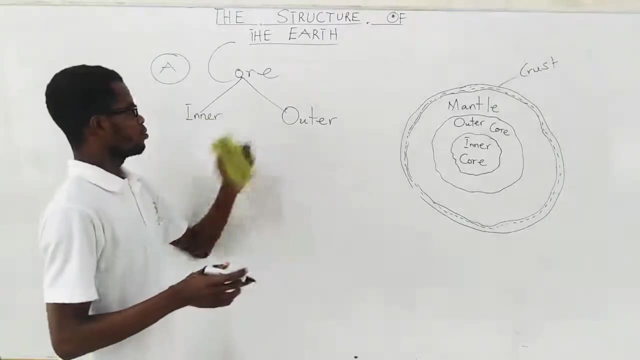 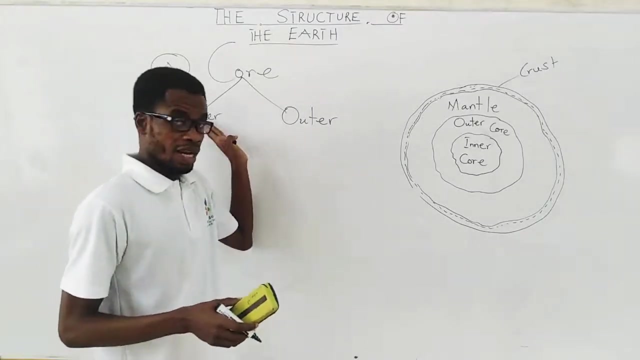 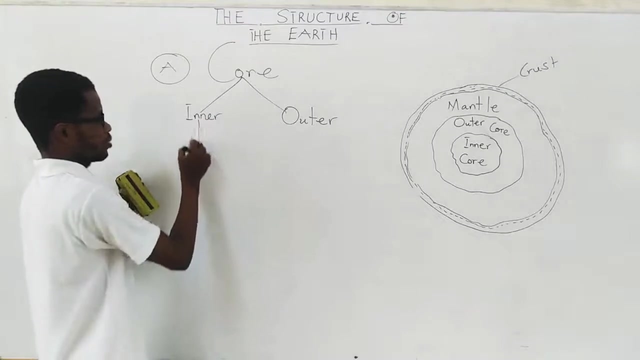 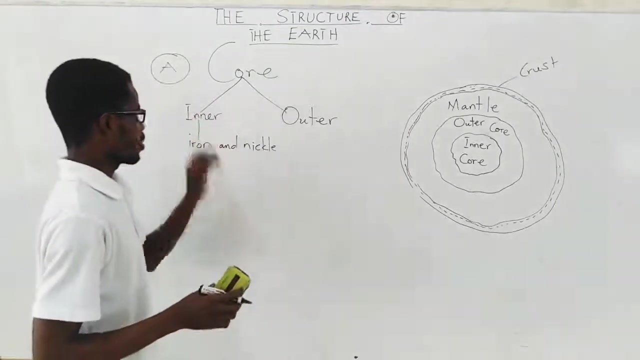 or has two parts: inner and outer. what? why do we have to divide the core into two? because the nature of this layer or sub layer is different from this particular sub layer. so what do we find here? we find iron and nickel as a major element in this inner most part of the earth. so this is the 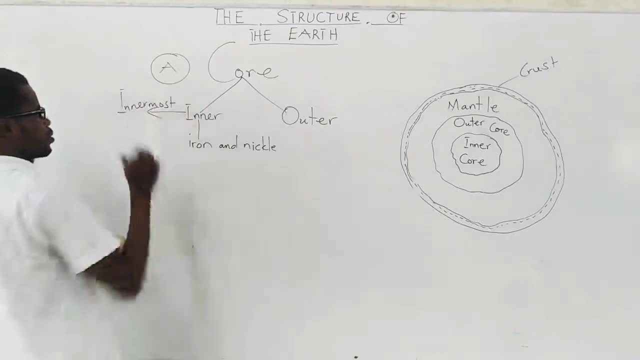 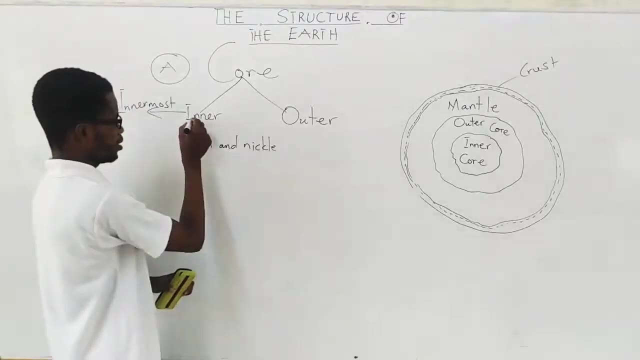 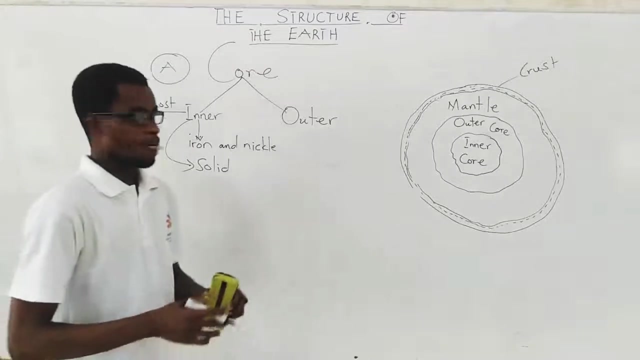 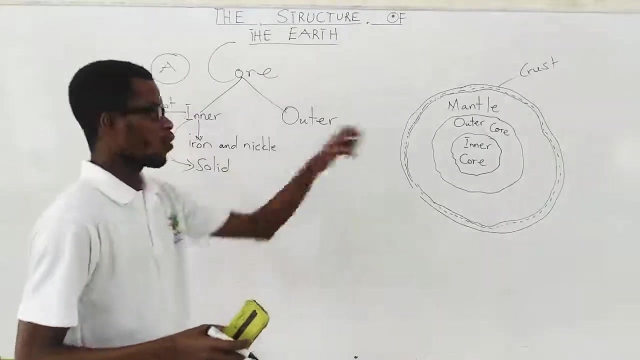 inner most part. so we need to find the inner core of this inner core, the inner most part. so iron and nickel found here, thereby making the inner core solid in nature. solid in nature, but there is heat here anyway. but this is the most interior part of the air. let's come to the outer core. the outer core, the core of the air, is the core of the earth. 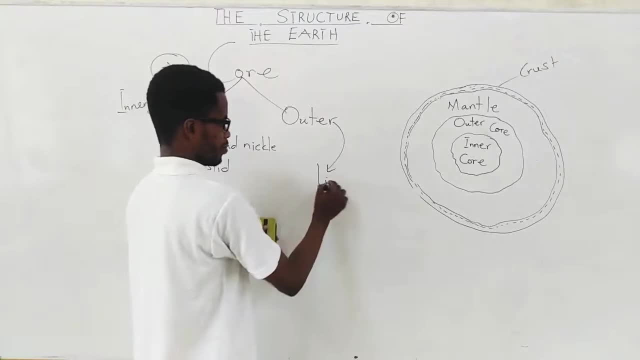 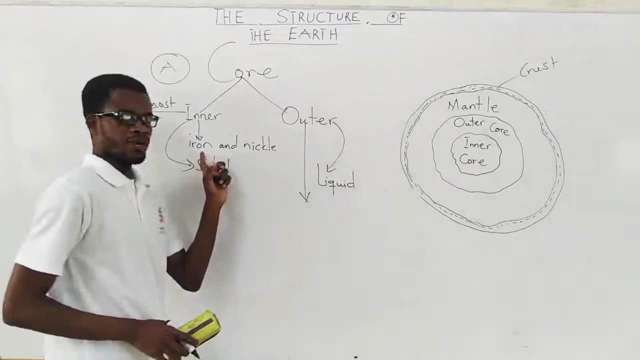 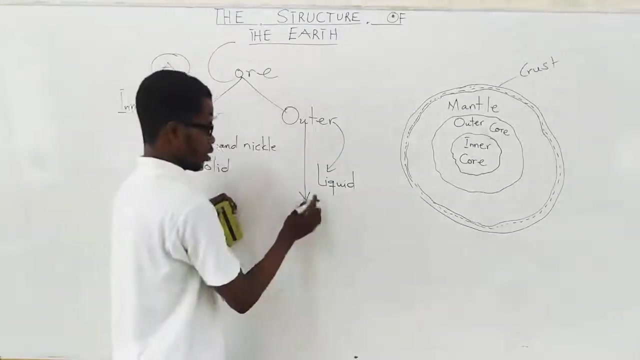 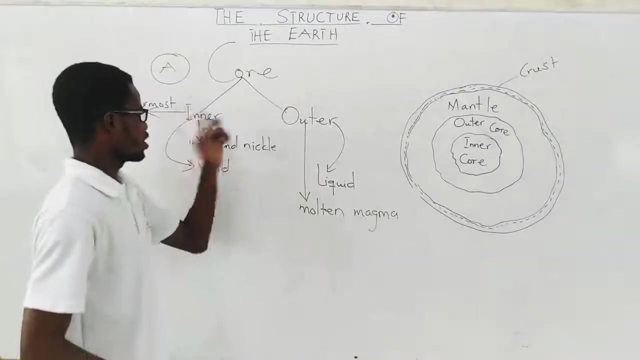 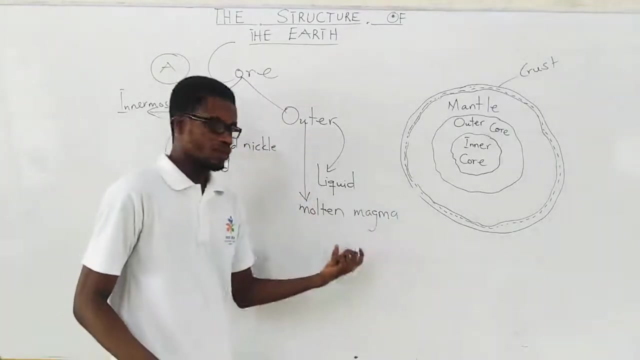 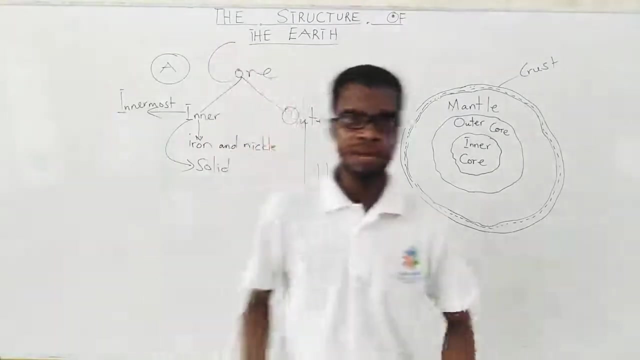 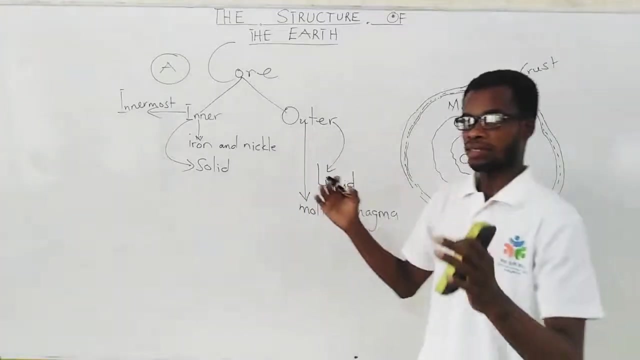 It's not solid but liquid. So what substances are found there? So we may find these substances there, but the liquefied nature or the liquid nature of the outer core makes these elements to be melted, to become what we call molten magma. So inner core is solid, outer core is liquid due to the presence of molten magma. So if you are being asked to describe the core of the earth, you have to state that the core of the earth has two parts or layers or sub layers, namely the inner core and the outer core. 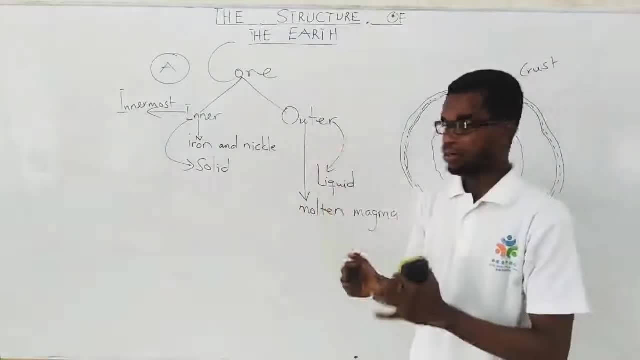 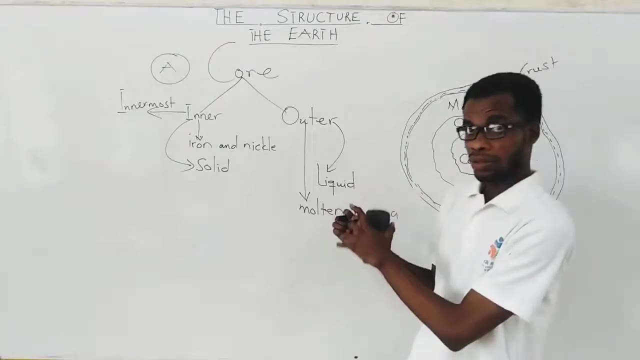 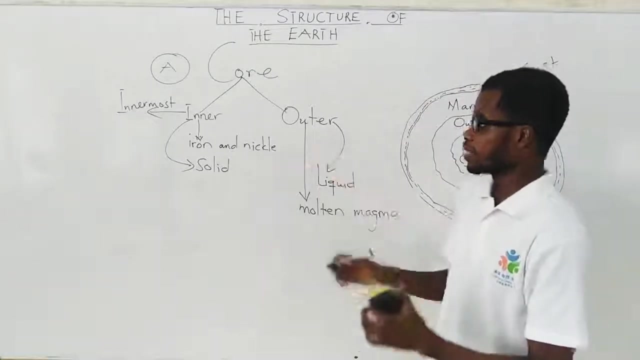 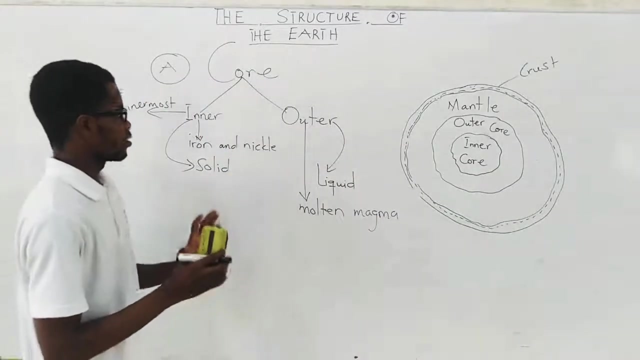 The inner core is solid. It contains iron and nickel, thereby making its nature solid. However, the outer core contains molten magma, and the presence of the molten magma makes the outer core liquid in nature. I hope this explanation makes it clear for all of us. 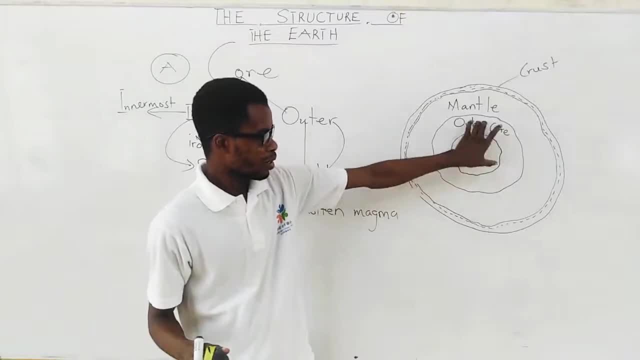 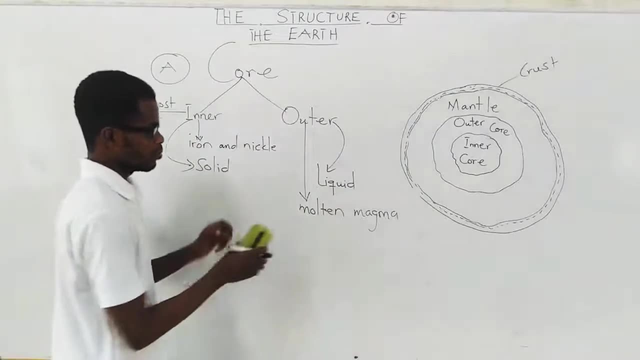 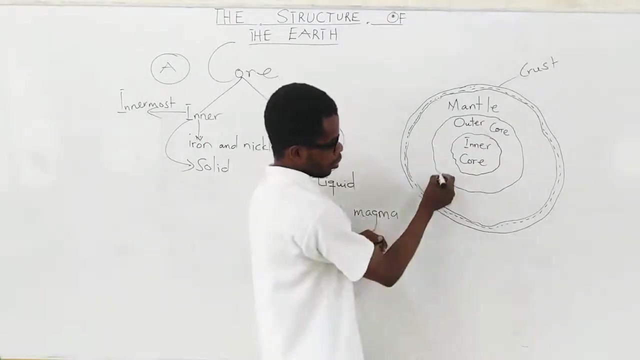 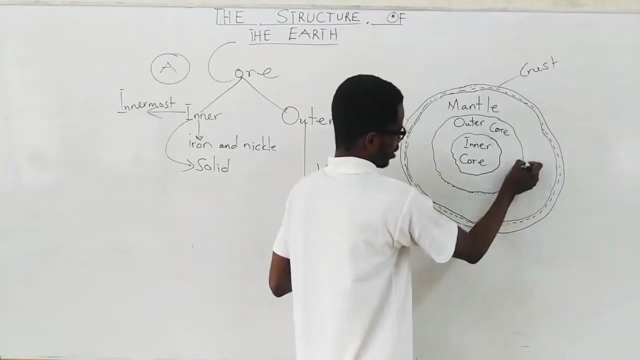 So this is the part we are talking about. So solid liquid. Now we can move to the mantle. We can move to the mantle, But before you cross from the outer core to the mantle, a man called Benno Göttinger discovered a layer, a thin layer, which some people also describe as a boundary. 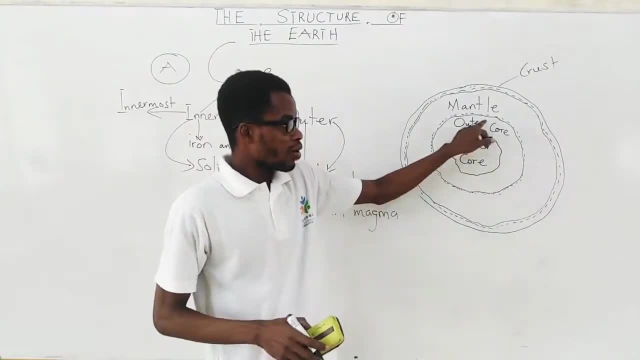 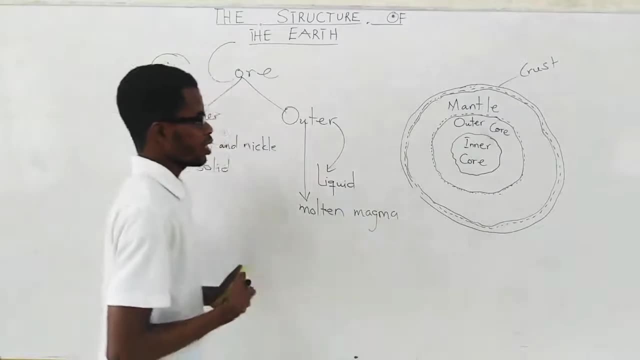 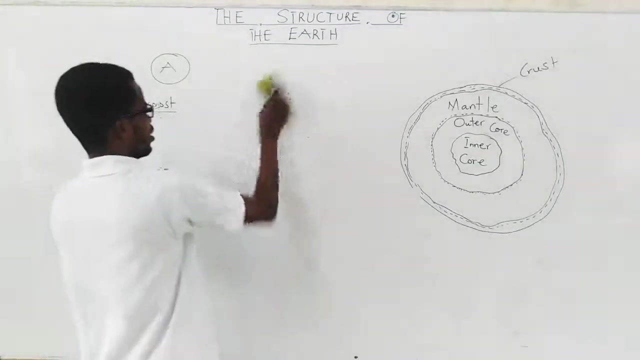 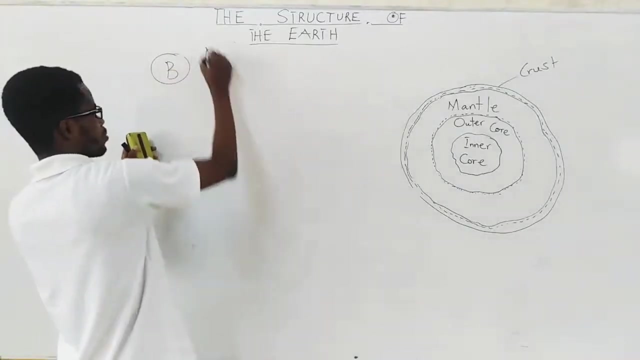 A boundary, A boundary Between the outer core and the mantle, So you have to cross that boundary before you can enter the mantle. That's how special the mantle is, Okay, So now let's get to the next layer. Let's get to the next layer. 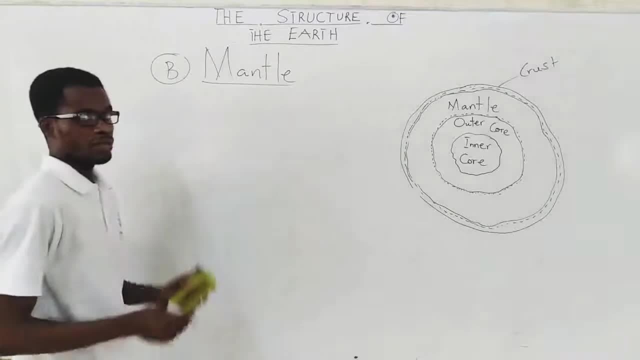 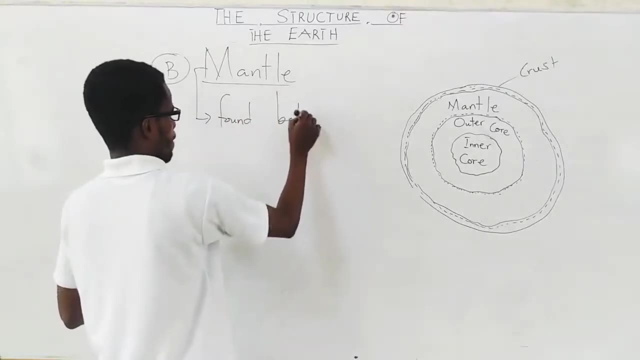 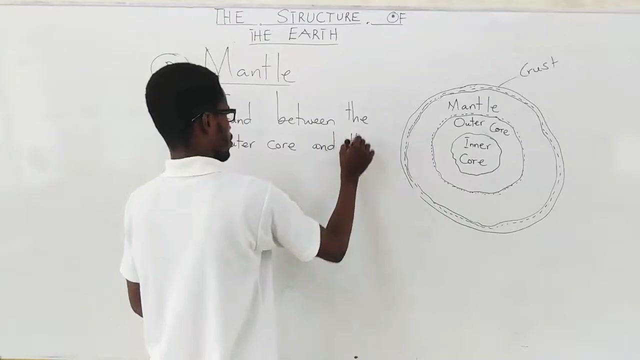 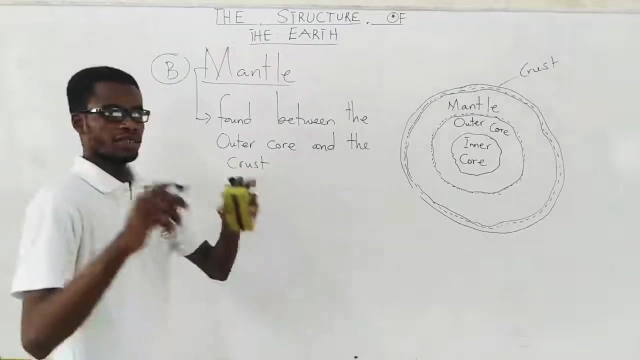 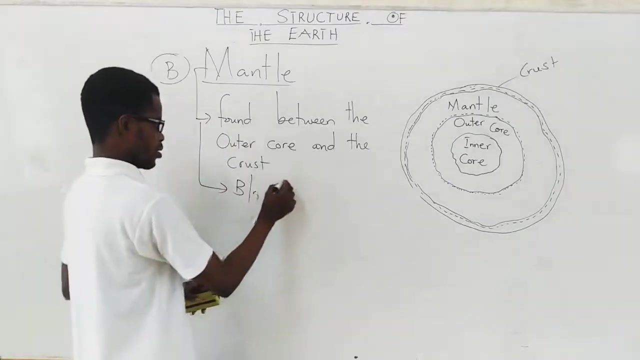 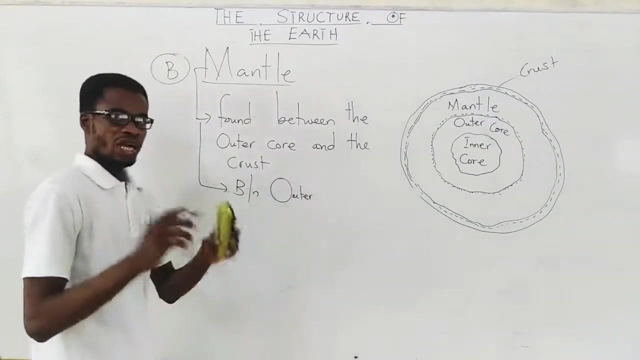 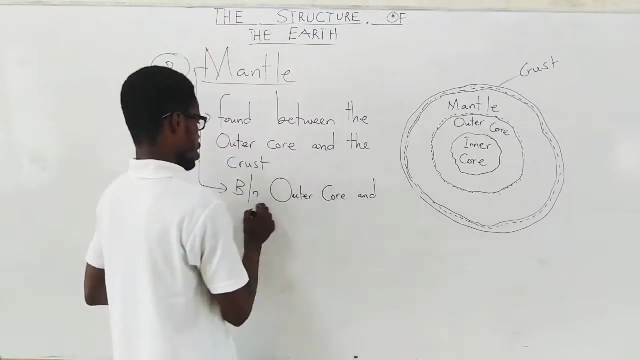 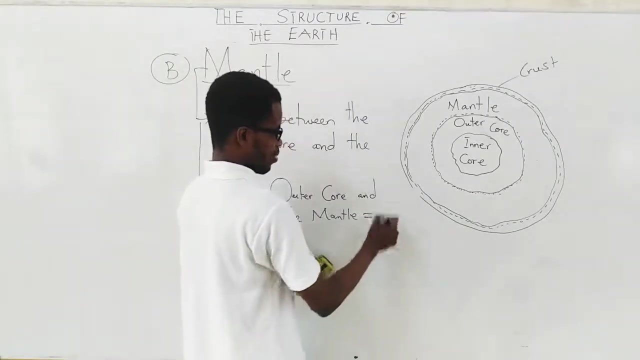 B, mantle. Okay, So the mantle is found between the outer core and the crust. The outer core and the crust- Okay, So let me do this: Between… Between the outer core… And And the mantle… we have the thin layer or the boundary that separates them, and that is called Gartenberg. 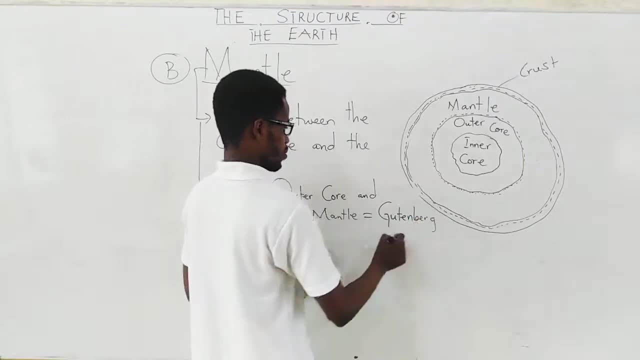 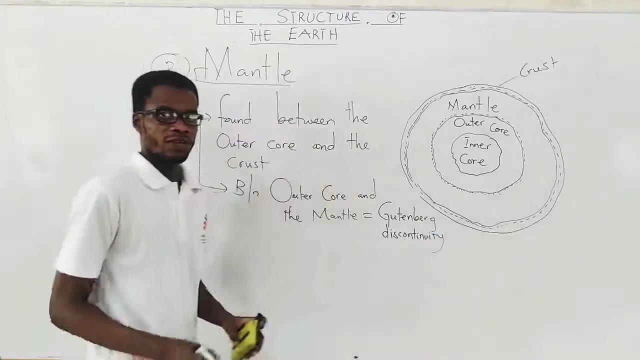 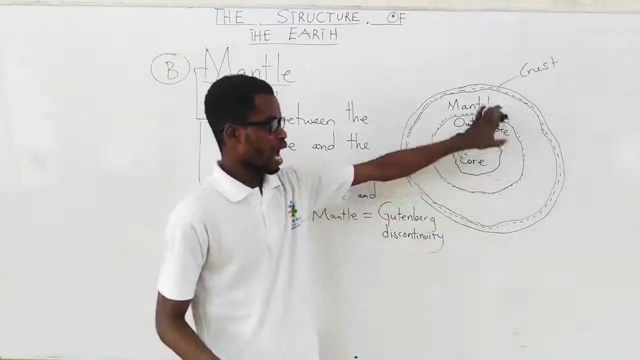 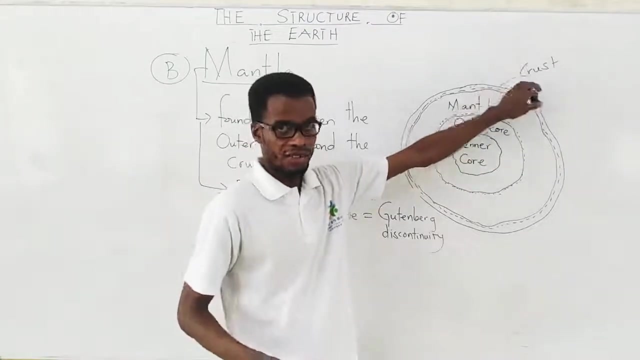 discontinuity, Gartenberg discontinuity. so that is the thin layer or the boundary that separates the outer core and the mantle. okay, so if we move from here you cross that boundary, then you get to the mantle, from the mantle. before you get to the surface of the egg, where we are, that is a crust of. 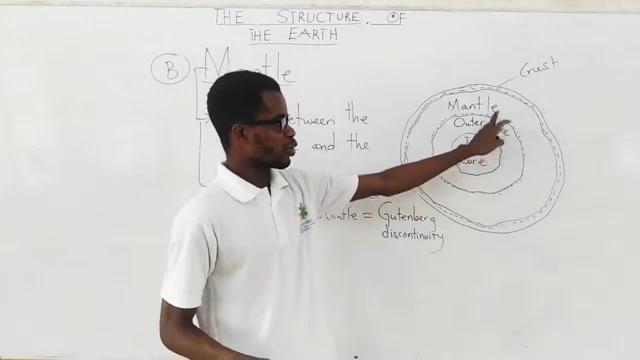 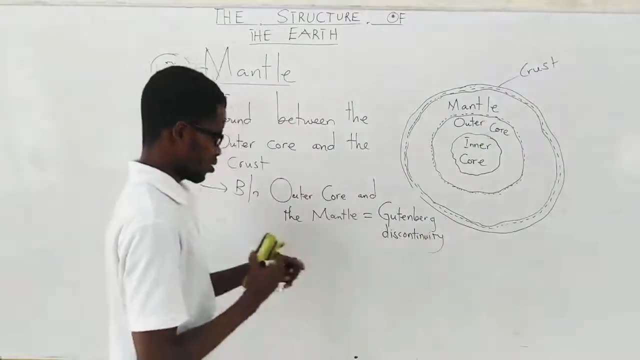 the egg, then you have to cross another boundary again. you have to cross another boundary again before you get to the crust that one was discovered by. so this was discovered by. I did say the name is Benno Gartenberg and this is the first one that I discovered 10 years ago. so let's just say: 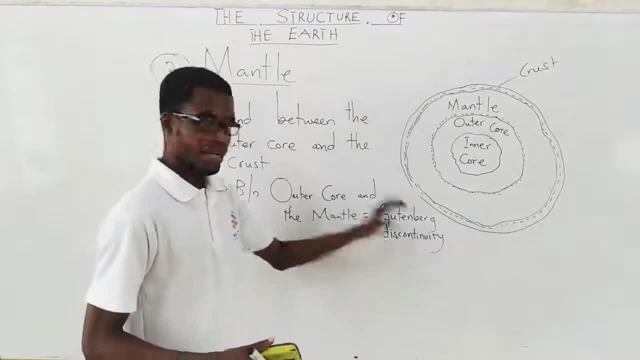 15 years ago now. the first was first discovered because importance from the trainee, I think. after what was, do you know in university school you were after do you work as a professor in shadow. It was named after him. It's an American-German who discovered that boundary, or that layer. 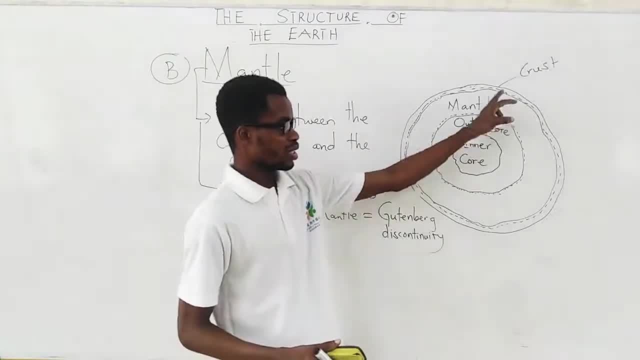 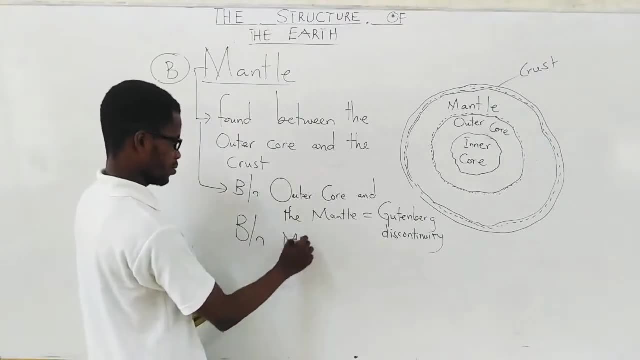 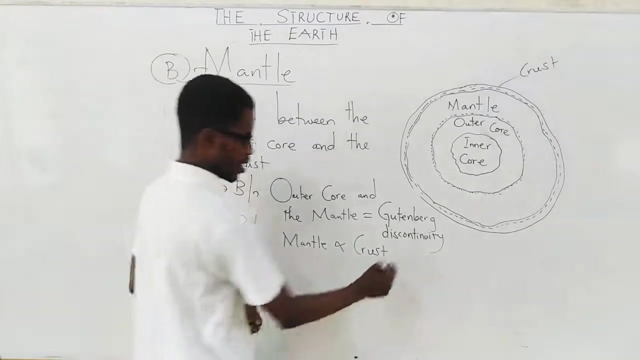 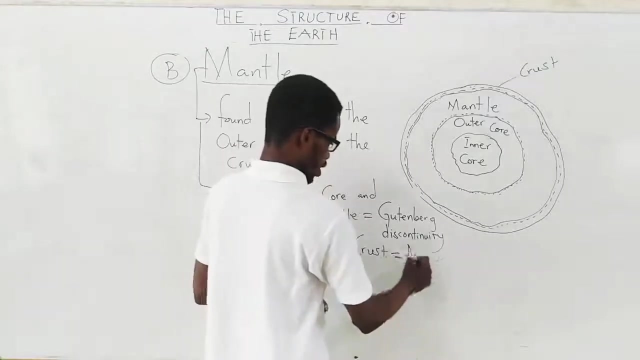 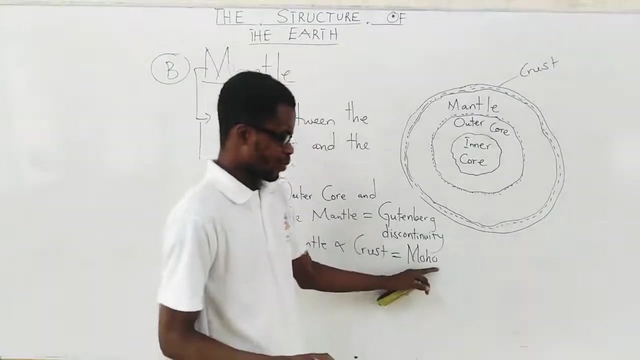 Then we look at the one between the mantle and the crust. The one between the mantle and the crust, We have the Mampayana-Mohoro visit. So, in short, because of how jaw-breaking the name sounds or the name is, we make it just short. 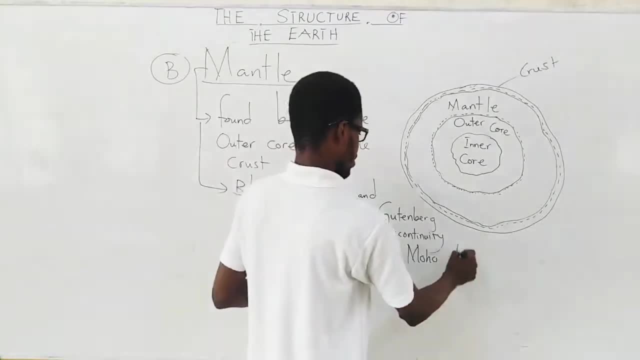 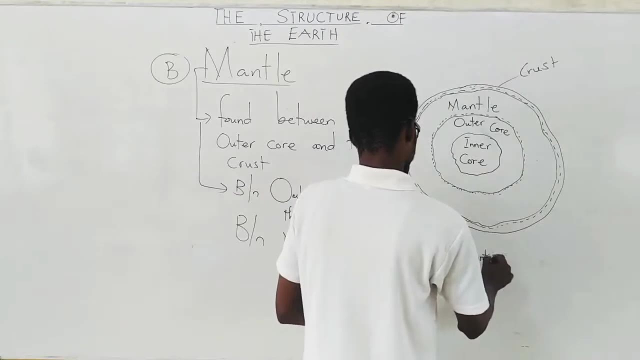 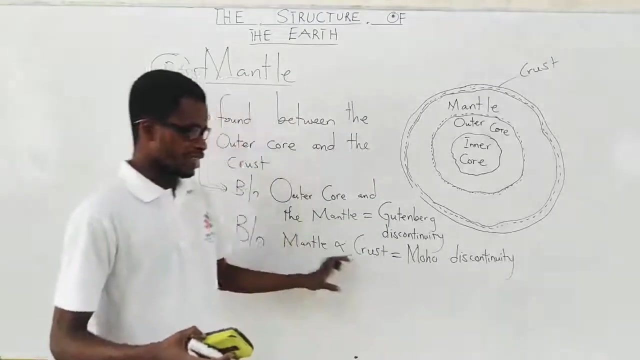 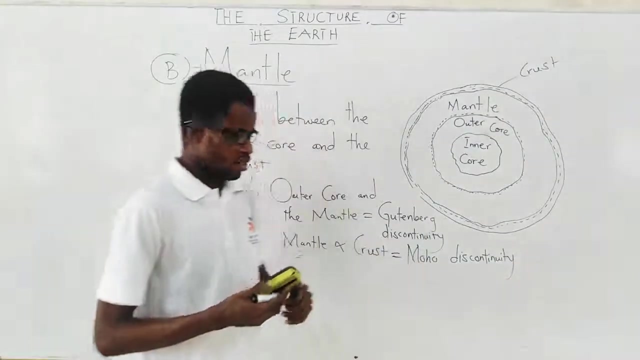 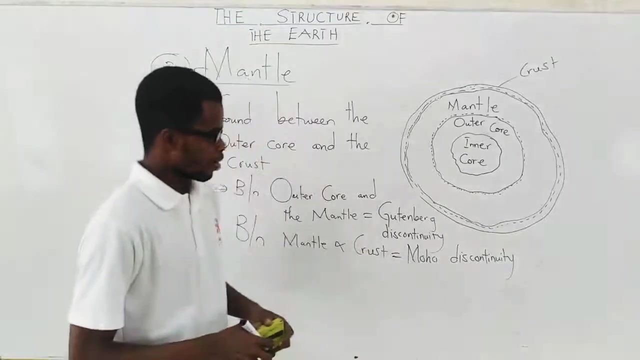 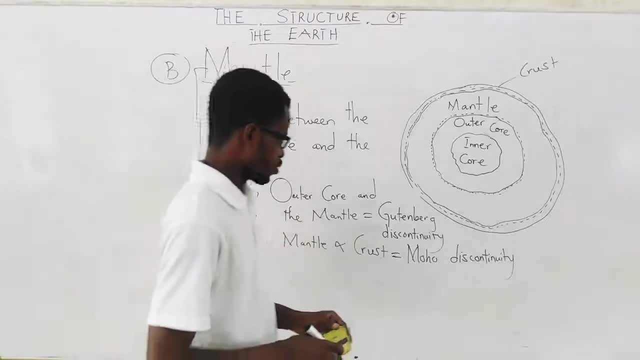 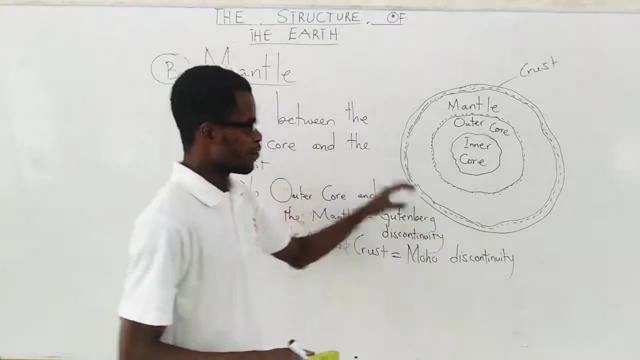 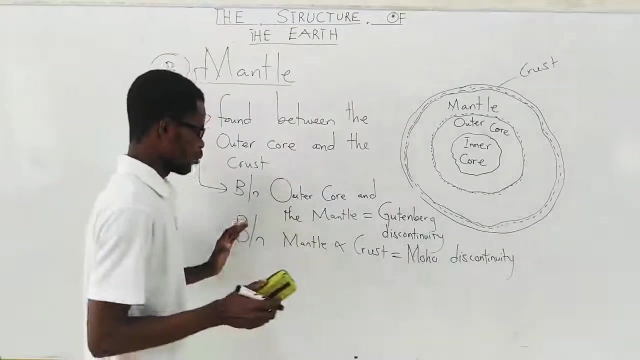 These people have done a great job trying to know what the Moho discontinuity is, What is actually inside that part of the earth Before you get to the crust. that is the boundary you have to cross from the mantle. Now we know this about the mantle. 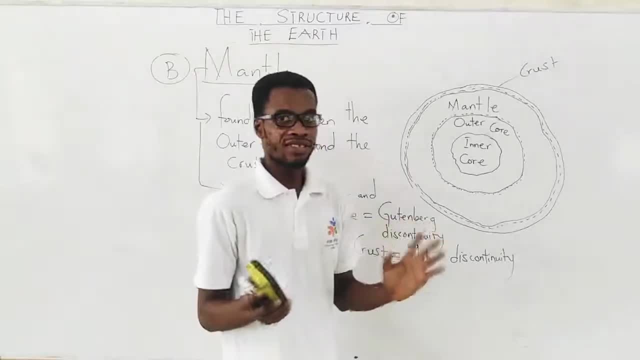 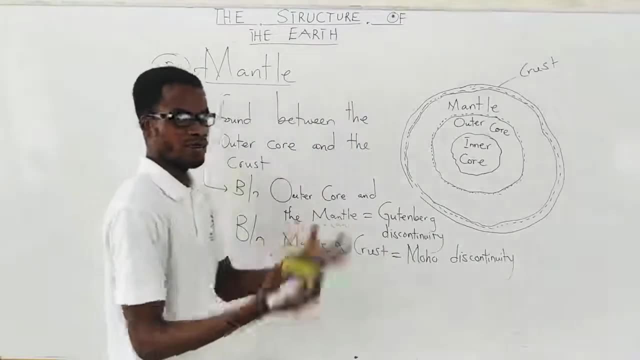 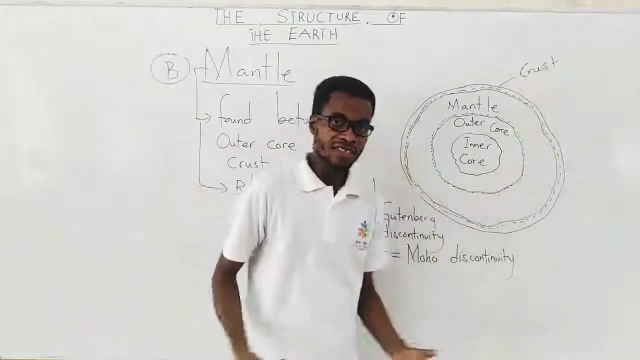 I think at this level it is sufficient. So let's get to the crust where we live. The crust where we live, Where human activities take place, Because this surface or the crust is supposed to The sun's heat, light, the atmosphere and every other thing and human activities. 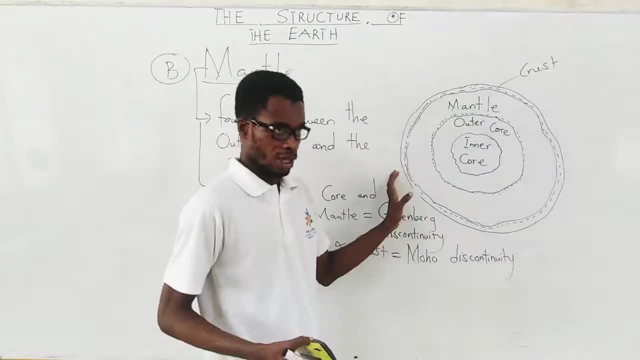 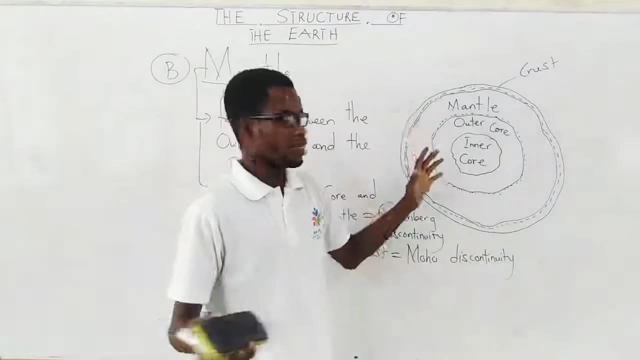 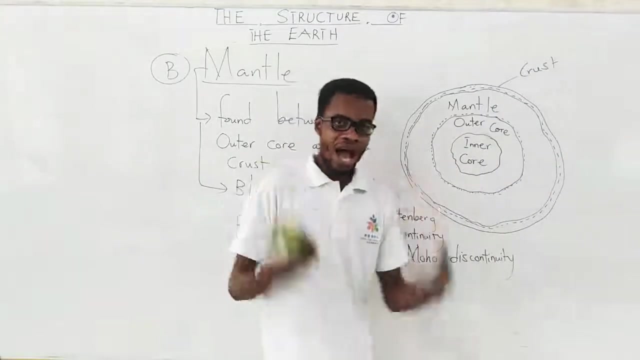 It makes this surface to be very hard. So softer layers are down the crust, But this surface, because it is exposed to the atmosphere, there is always pressure on the surface of the crust, Therefore making it the hardest layer of the earth. 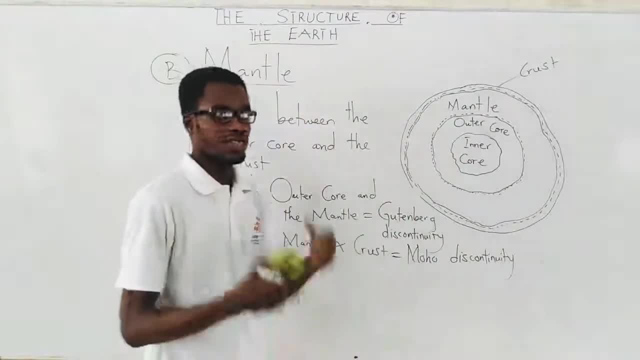 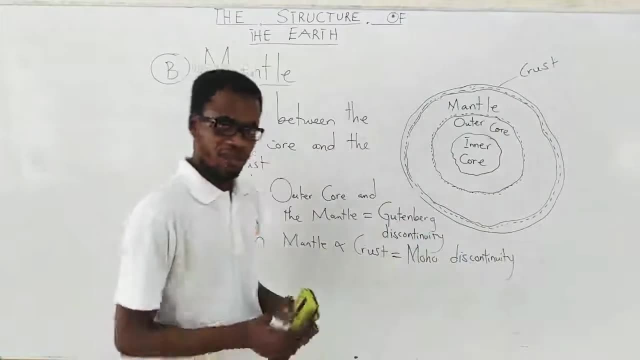 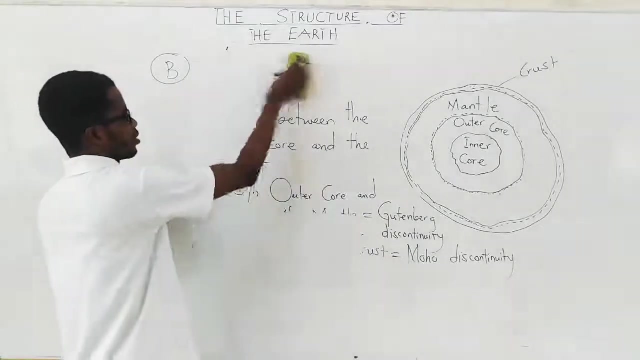 The earth layer. The three major layers we have already mentioned. It is the hardest And because it is the final layer at the top, we also describe it as the outermost layer of the earth. The outermost layer of the earth- Okay. 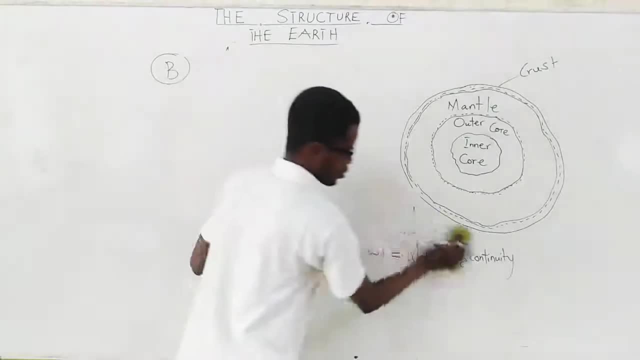 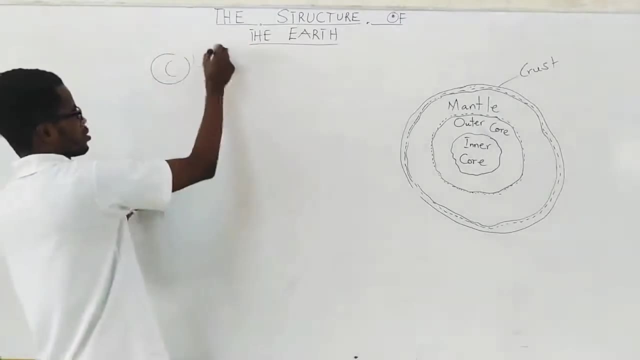 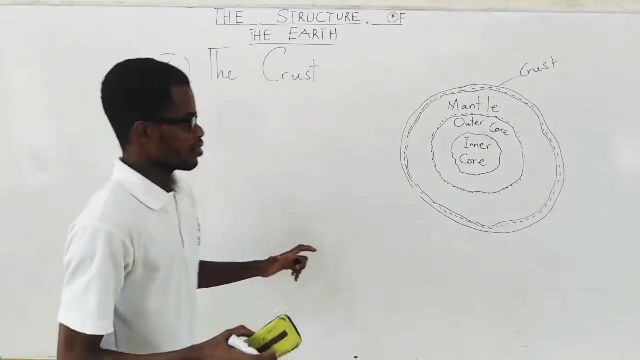 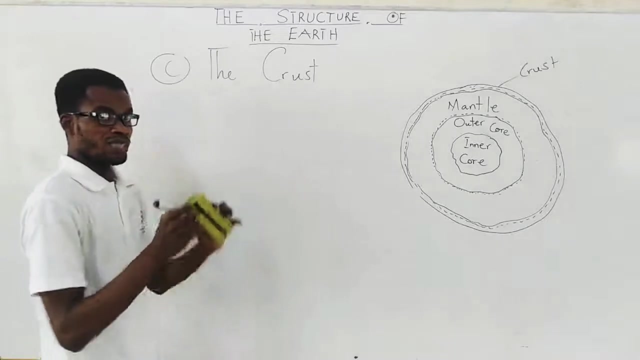 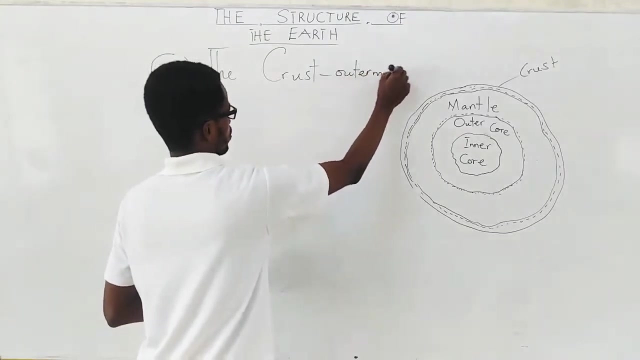 So we move to the layer C, Which will be outer layer And outer layer of the earth, The crust, The crust, The earth crust, The earth crust. Let's go into that Now. the Earth Crust is, We say, the outermost and the hardest. 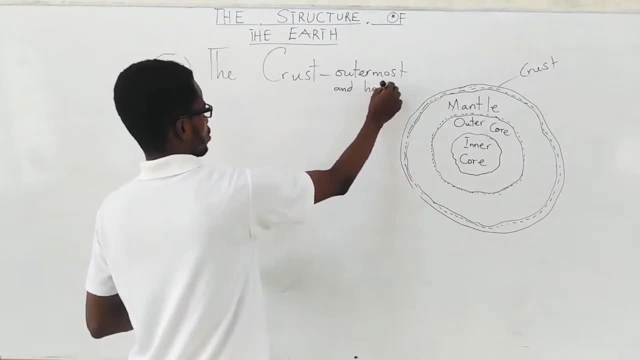 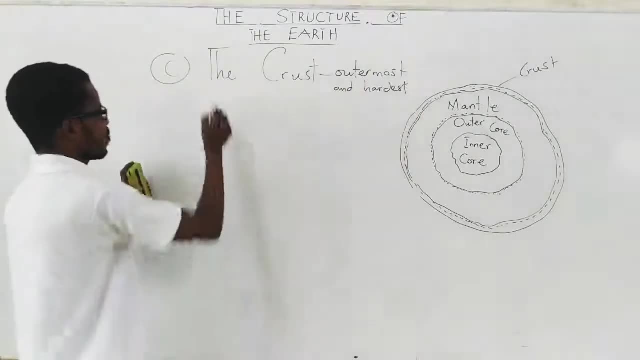 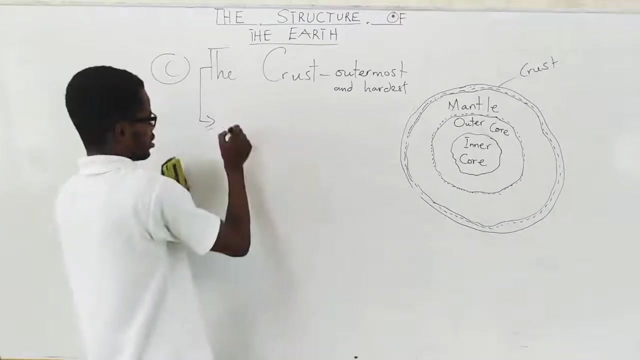 So take note, because when we are delivering there is a difference. Okay, notes, because we are describing it. we need to indicate that. then what else can we say about the head class in terms of eight parts? so let's begin with each layer. it's so compact, it's so huge. 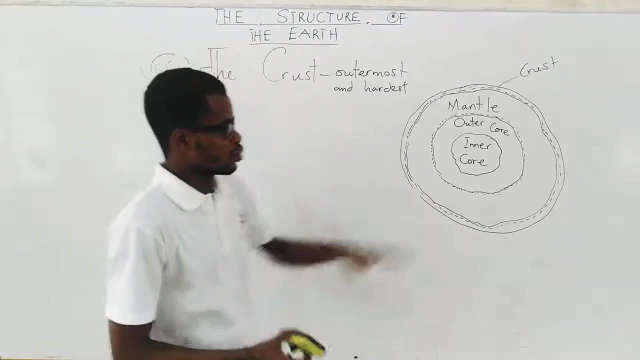 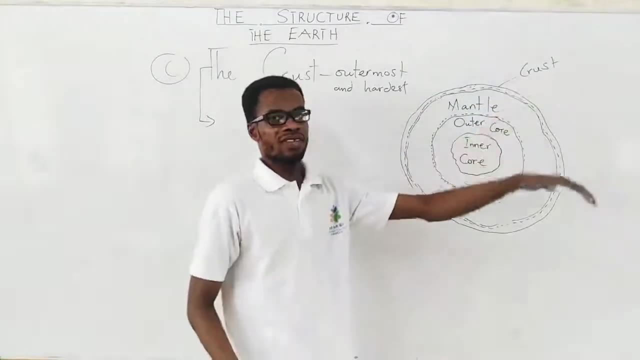 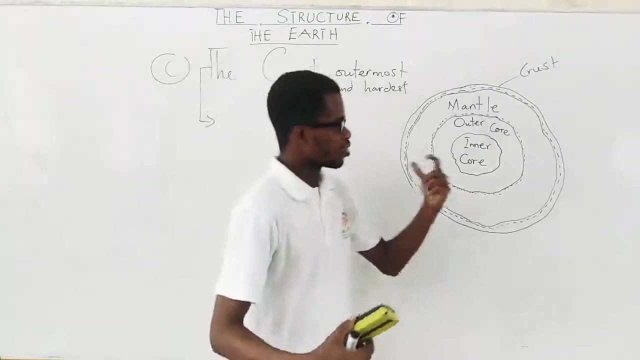 that you need. the diameter is very fast, so you need to dig deep before you get to the mantle if you are on this surface, so you don't just take off the first cover or sand or soil away and then you get to the mountain. it's very thick, okay, why? because part of it even leaves a foundation for. 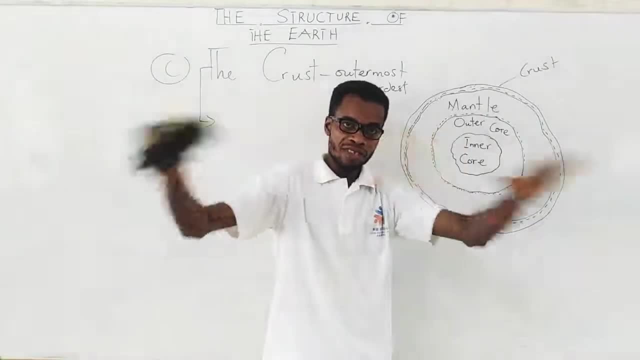 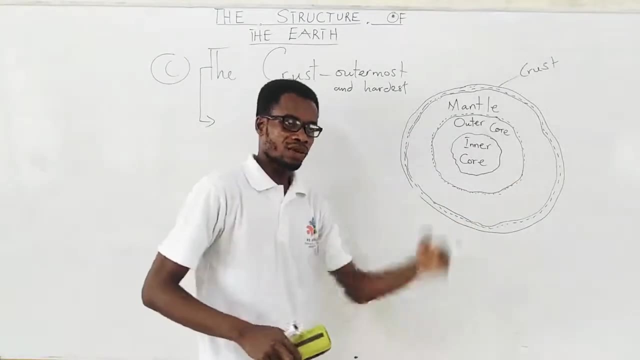 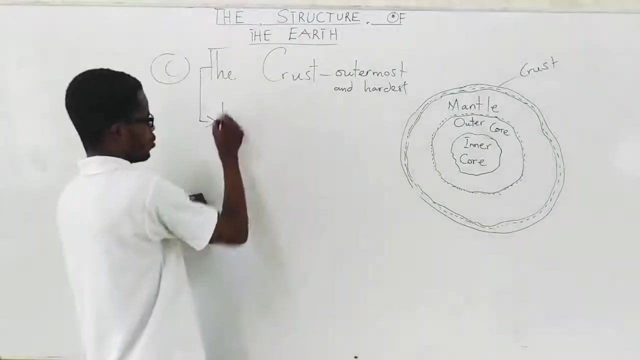 the ocean. for the ocean, that is the water covering the surface of the earth. okay, so we'll get into that and see that part that lays the foundation of the path that the ocean of the earth is found on. okay, so look at this. it also has sub layers. 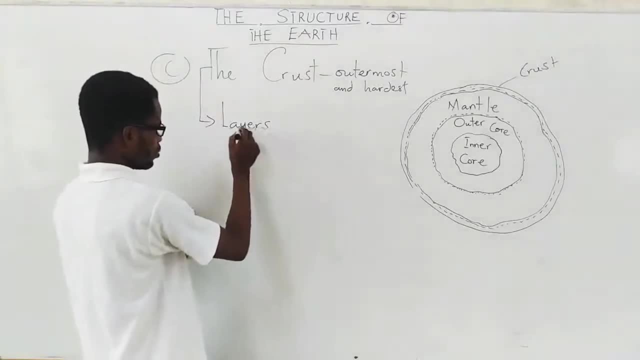 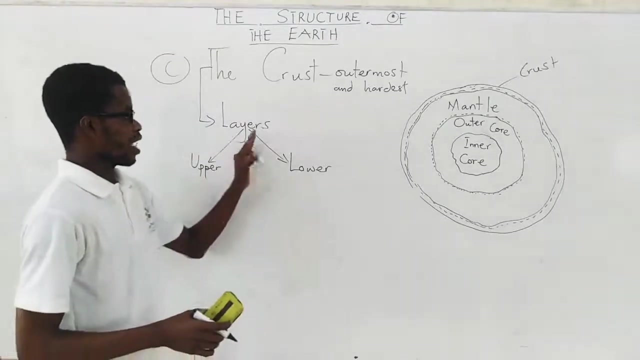 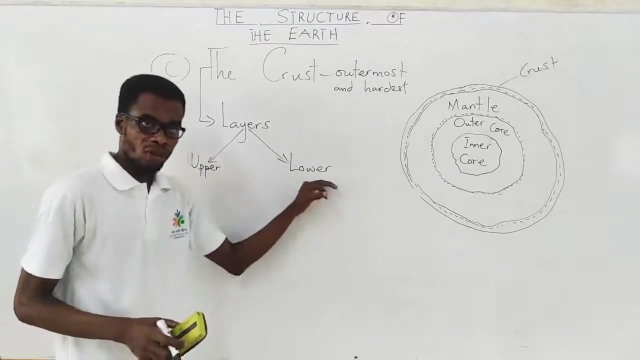 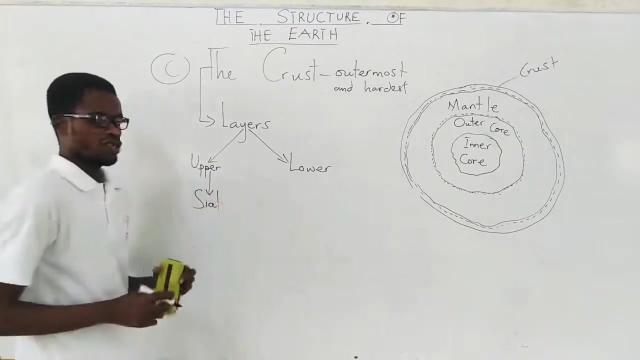 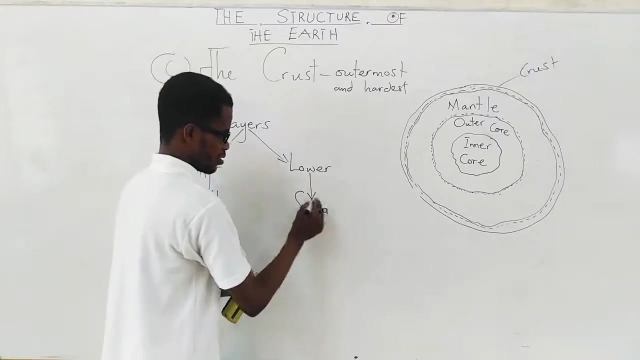 with eight layers. we have the, we have what we call the upper layer and the lower layer. the crust has two major layers: the upper layer and the major- sorry, the upper layer and the lower layer. okay, the upper layer is described as it's technically called, sial, while the lower layer is described as a sema- sema. 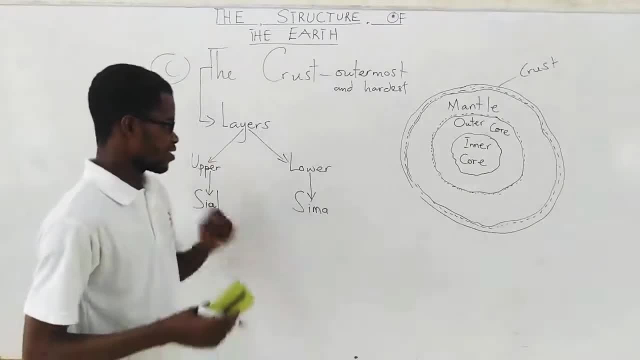 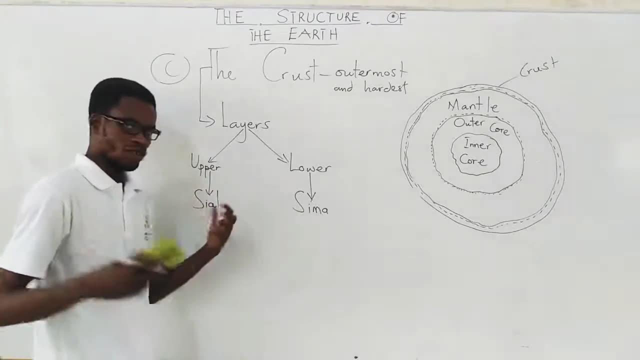 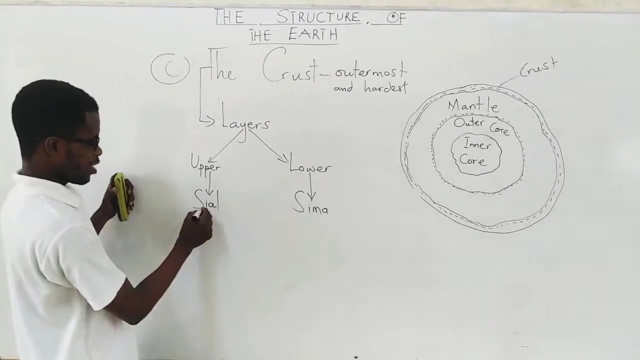 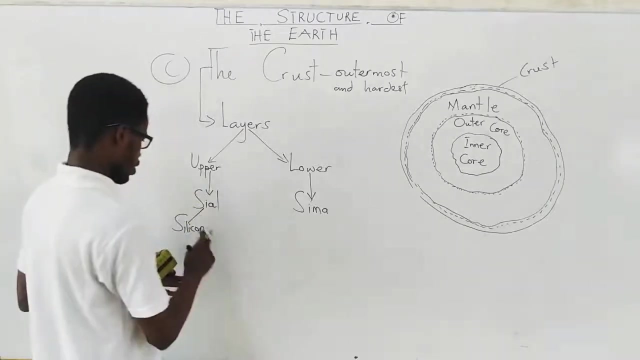 so if we know this is the sial and the sema, then what substances are found here? so this name actually came out of the combination of two elements: combination of two elements. so sial is s, i represents silicon or silica. okay, so silica rural, then the al alluvium. 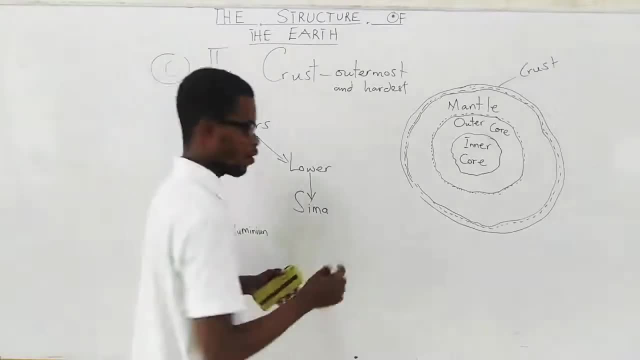 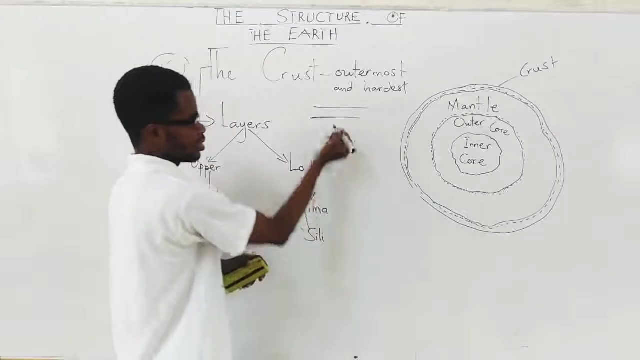 that is the composition of the sial, then the composition of the sema. we have, yes, the silica again located in that part of the sema. that is the composition of the sial we have of the lower layer. so if the crust is built like this, the top most part or the top part is a 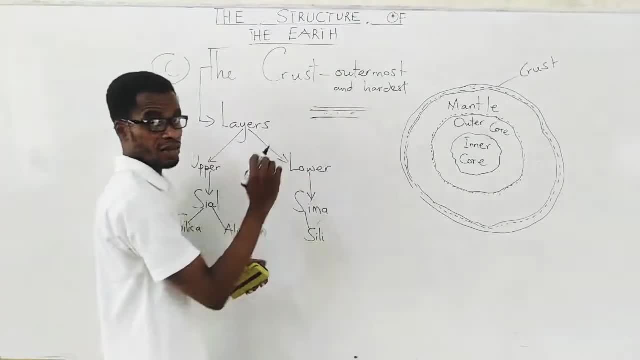 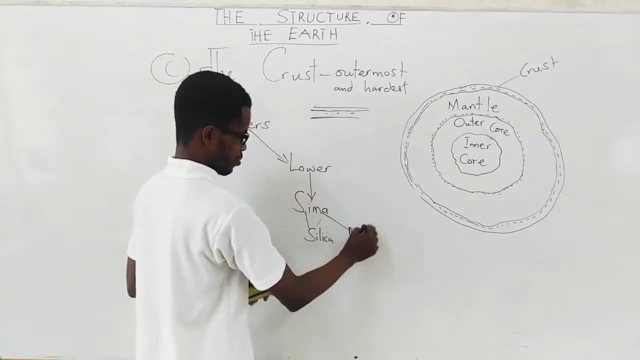 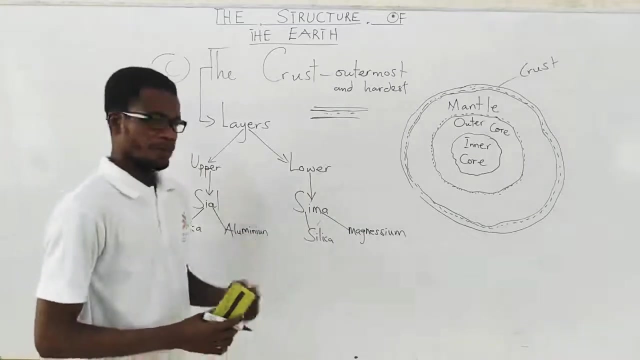 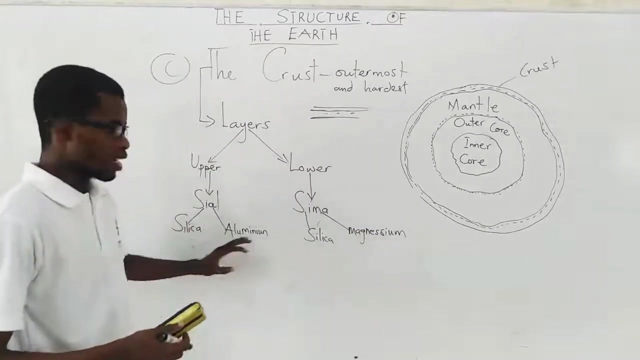 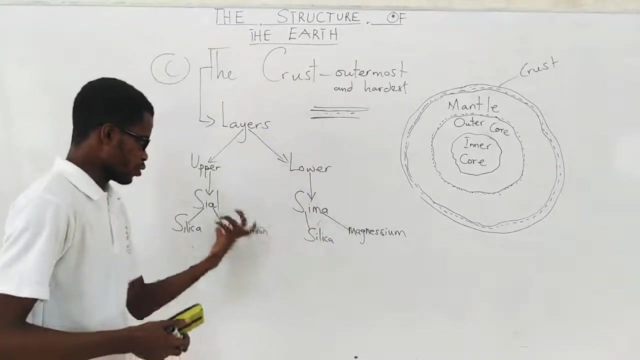 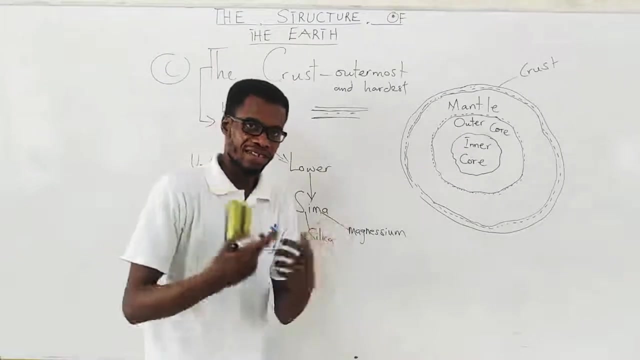 cr and the down part of the crust is a sema- okay, so the silica again. and then here we have magnesium. magnesium, okay, as the um. so if you are able to identify this, it is easy for you to also identify. how do you know for the students who want to maybe connect letters and try to match them and get it? 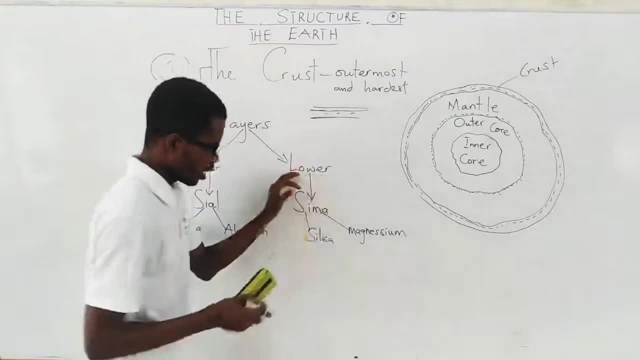 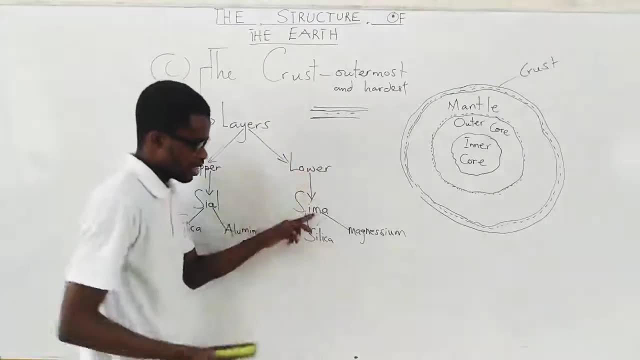 easy um. look at the lower. when look at the lower, there is a w in the lower, so the w. you look at this. when you turn it upside down you get an m, the m in the sema. so that will be a m here. so turn it upside down so you link the lower. 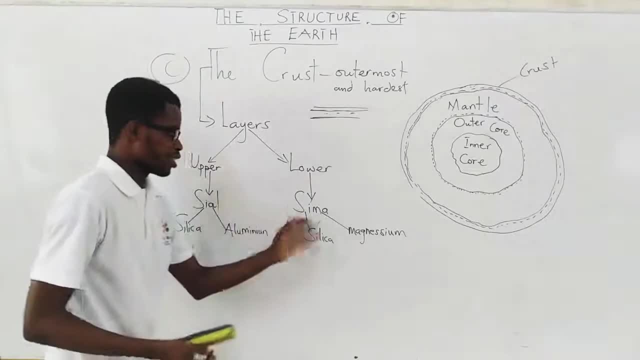 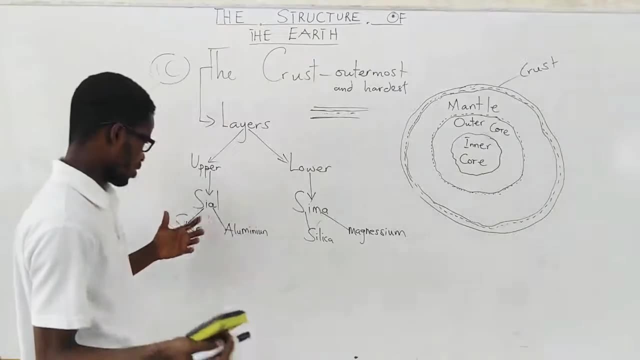 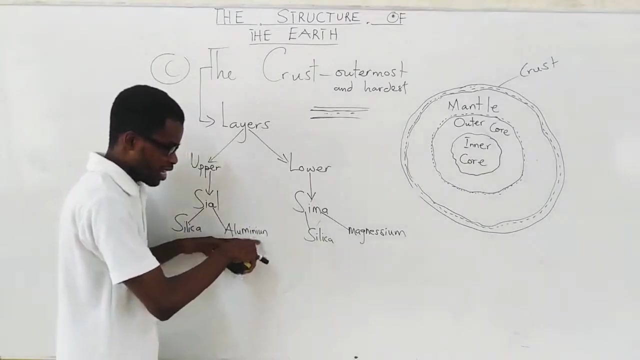 to the sema, then you can get the substances. then, if you know this, then you know that the upper one will be the seara. that's simple. that's simple, yes, or since we know silica and silica are common in both of them, then we look at the last element, or the second element. when you check the seana, the seana. 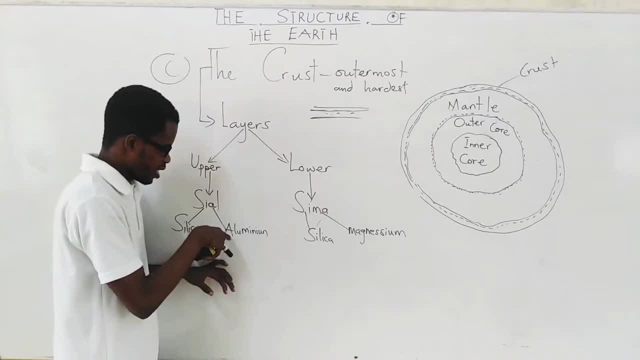 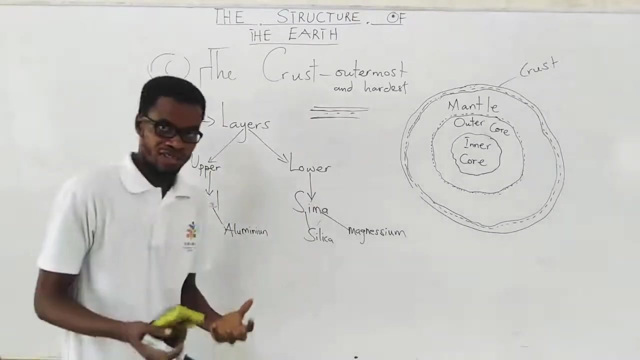 has was al okay, and that is the al also here. then you can match this u okay, the you here in aisle, nearly with the u here in upper, the u here in upper. if that can also stick in your mind easily, you can be able to do that. 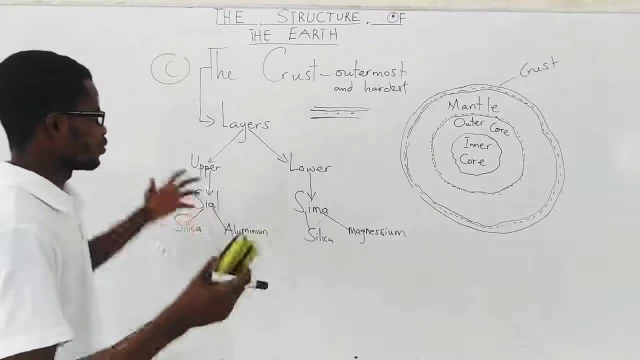 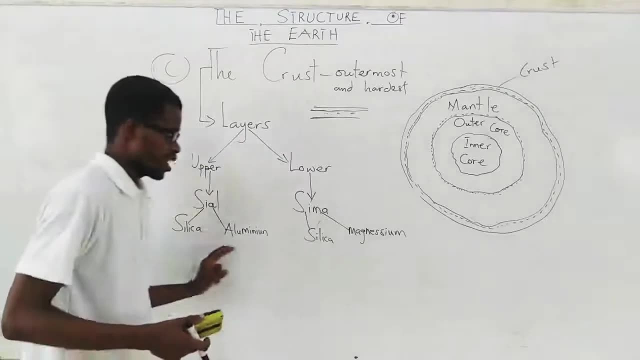 you can be able to do that. so what we have also banked in you. so that will not be very efficient. also, you will see, one of these elements you won't be able TO WORK ON THEM to know is that the layers of the crust are also two: upper and lower. the upper is sial, the lower 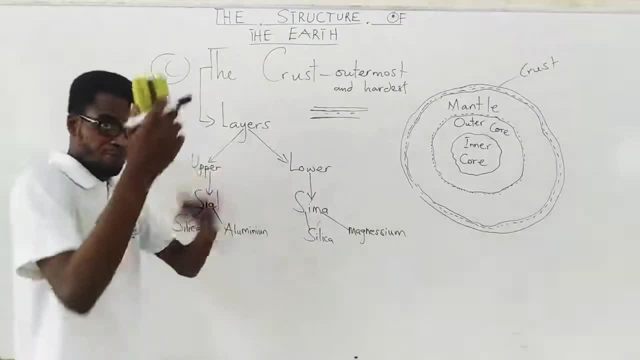 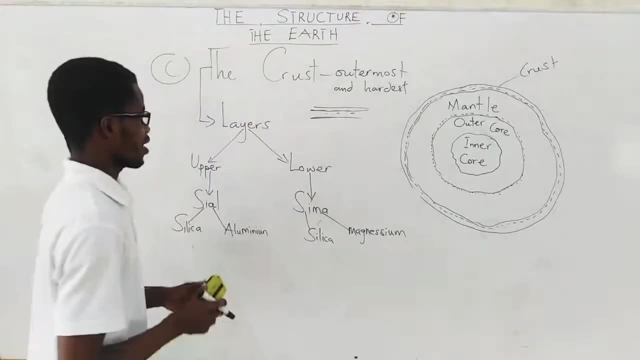 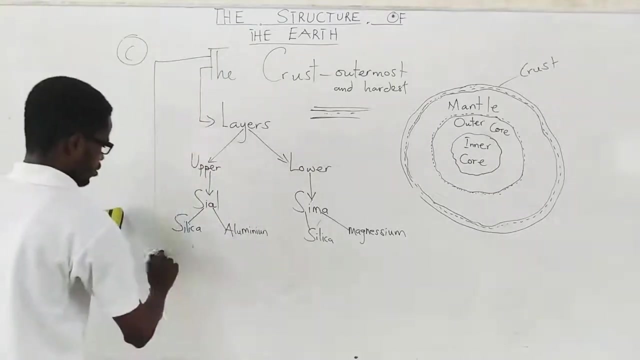 is sima. okay, so we are described. so you put all these sentences together and build a good description or a very detailed one for the crust. then, looking at the crust again, we can also talk about its part, its part. so when we bring this here, so the part of it, there are two parts of it. 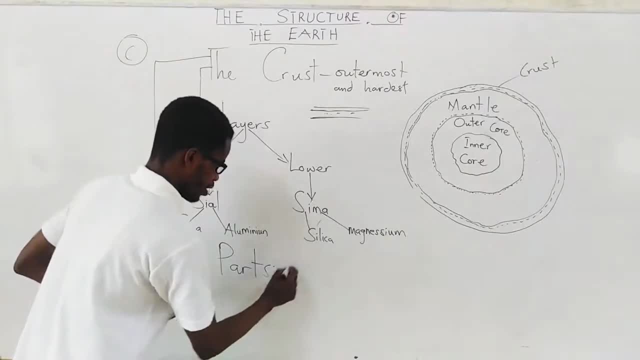 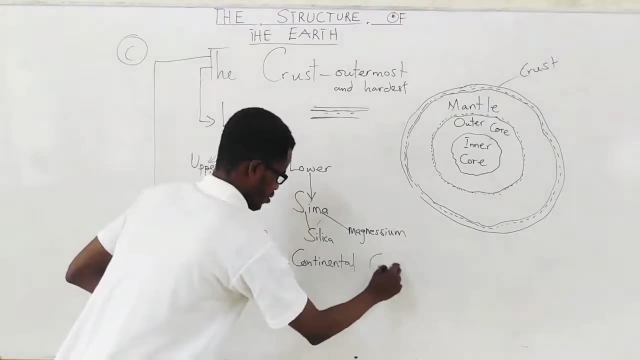 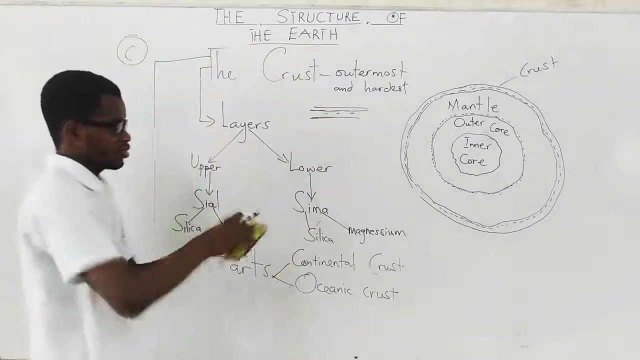 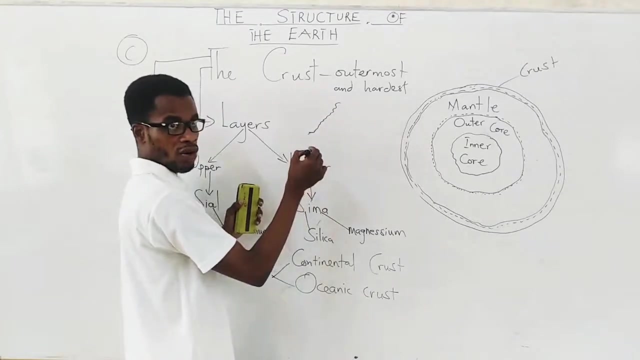 the parts of the crust, and we have the continental crust and the oceanic crust. these are the two parts, the layers and the part. take note the layers. they have that structure. so, if i should sketch this, if this is a coast or a coastal area and we have the sea, 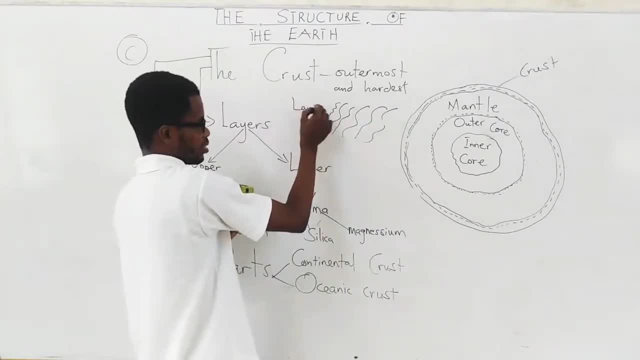 over here water body and this part is the land. so the part that is the dry land, where water has not covered, becomes the continental crust, where the parts that the water has covered become the oceanic crust. that means the layer. so if this part is a dry land, remember it has an upper and a lower, so the lower will stand down and become the oceanic. 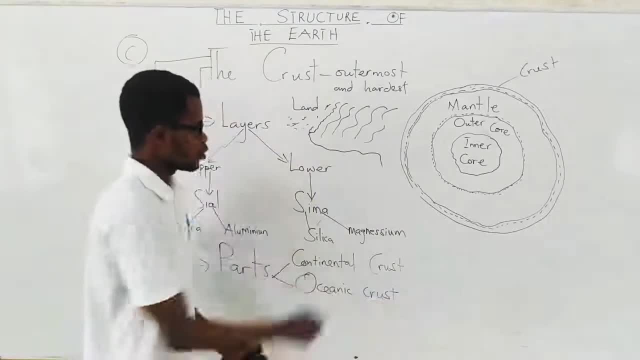 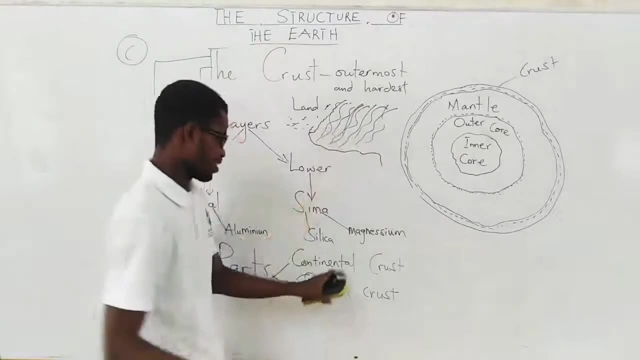 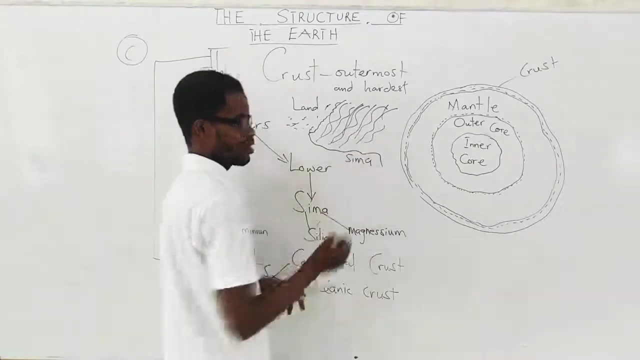 floor. that's what we describe as the oceanic floor. so the ocean of the earth is on the floor called the oceanic floor and that is a smmaker. that is the scene. so the ocean is on there. So Sima reaches this level and then you get to the top, So you have Sima all over this place. Then, when you move from the area where the Sima is located, you get to the area where the Siyah is located. 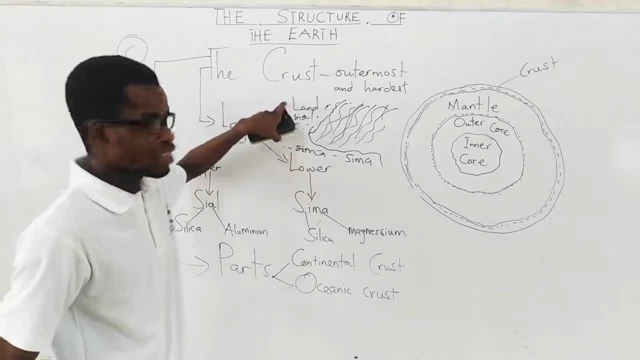 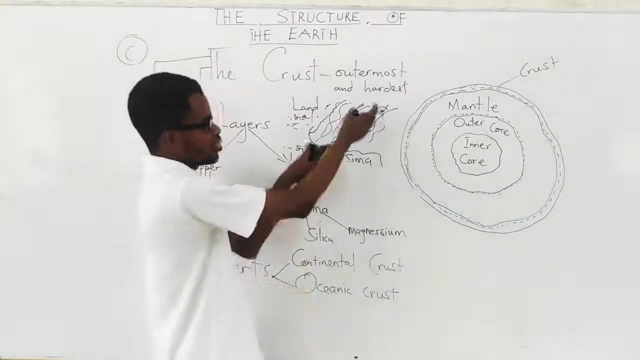 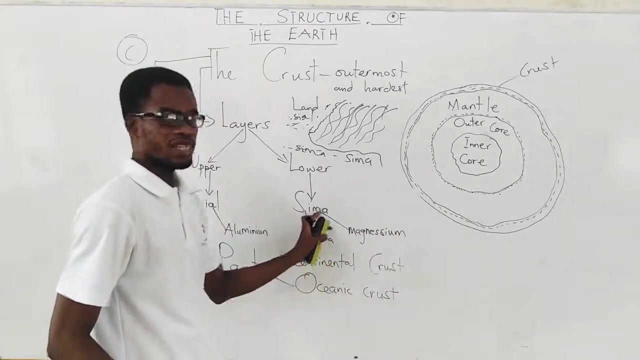 So the continental crust has a Sima and a Siyah, While the oceanic crust has a Sima and the water covers its surface. So water will take the place of the Siyah that we find in the continental crust. So take note, the ocean is on the oceanic crust, which is a part of the earth technically known as the Sima, or the layer of the earth crust known as the Sima. 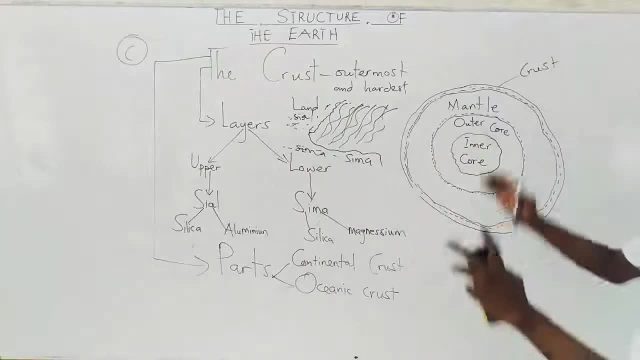 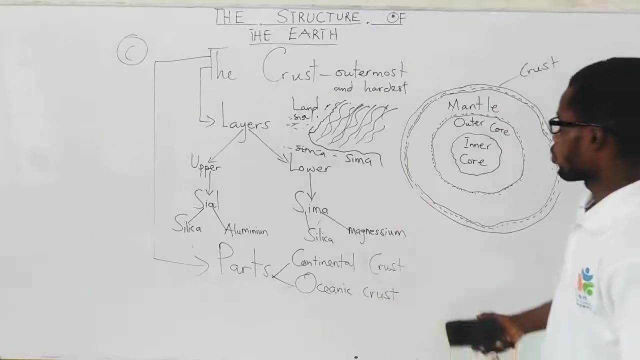 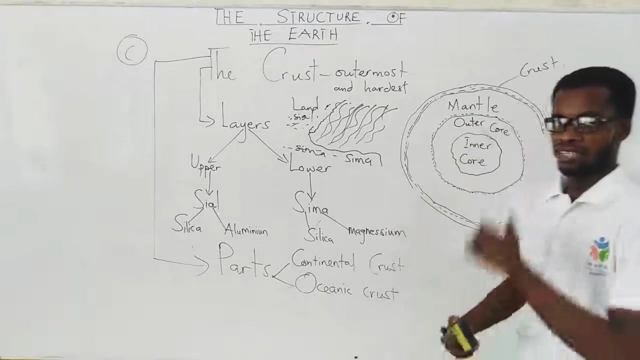 So. So if we know this demonstration, why can't we have a very nice description to describe the structure of the egg? So, by way of summary, we say: the structure of the egg has three major layers, namely the core, mantle and the crust. So the core has two sub-layers: the inner core and the outer core. The inner core is solid, the outer core is liquid. The inner core is solid because of the presence of the iron and the liquid. Then the outer core is liquid due to the presence of the molten magma. 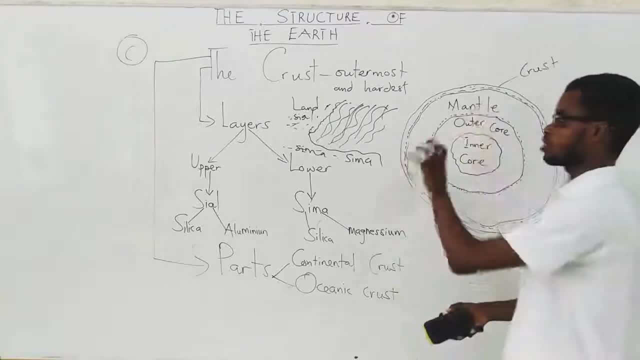 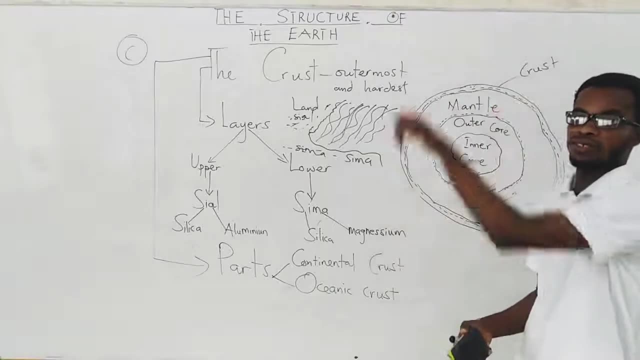 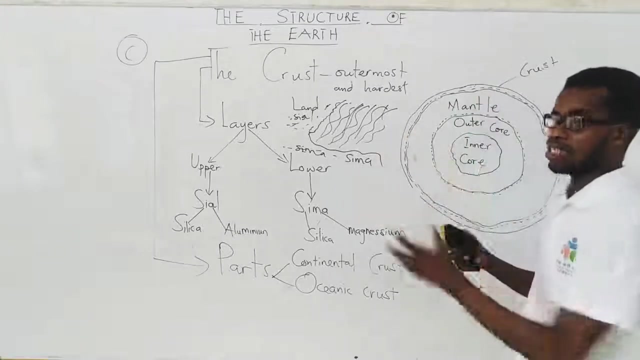 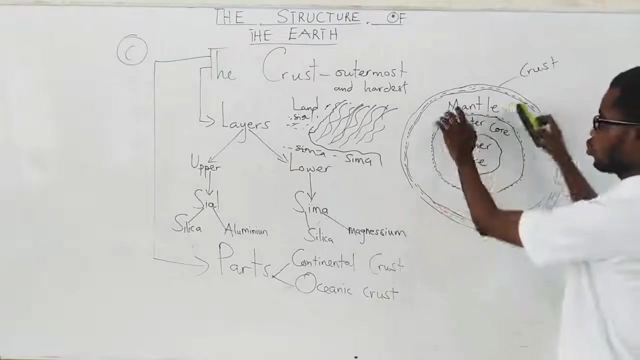 So the magma is here and that same magma is what erupts when you get a weaker portion of the earth layer and erupts or pops out onto the surface. So we know that we get into how mountains are formed. in our next lesson We move to the mantle and we say the mantle is so special that two boundaries separate it from the outer core and at the same time from the crust. 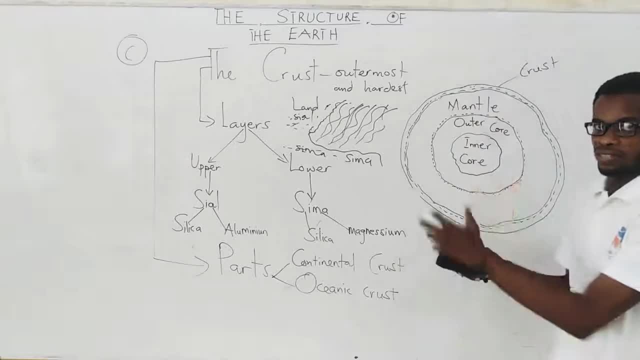 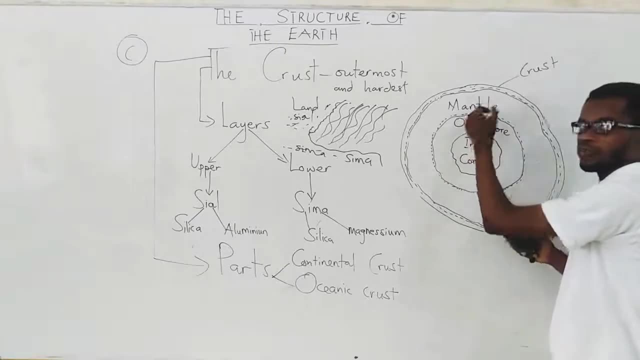 So the one that separates it from the outer core is the guttural discontinuity, So that one begins with the chin. So when you are starting the journey from the, So the innermost part, you really get the chin before the end. So the chin is the guttural discontinuity. 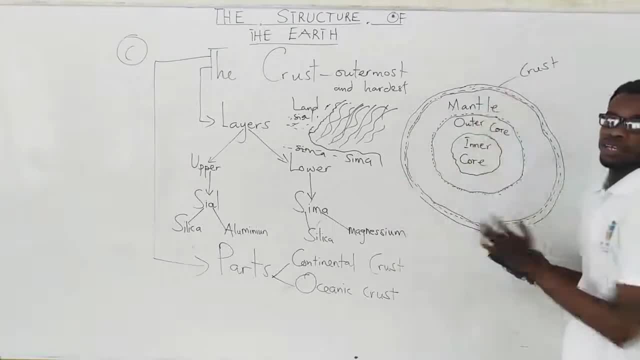 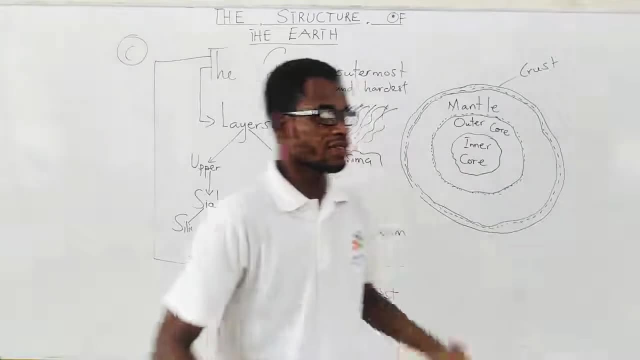 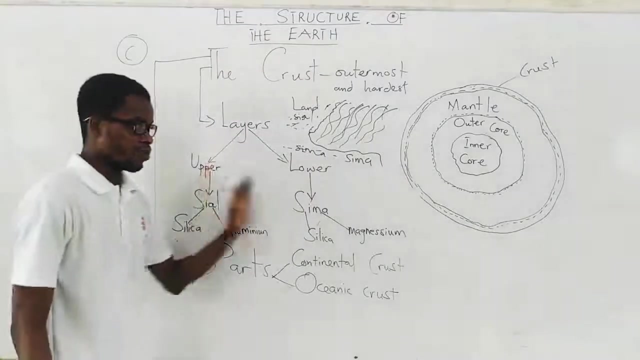 Then we have this part where the crust- before you get there, you need to cross that thin layer of boundary known as the mobile discontinuity. So that is what we said about the mantle, The crust. the build-up is here two layers: upper and lower. Upper is axial, lower is the sema. 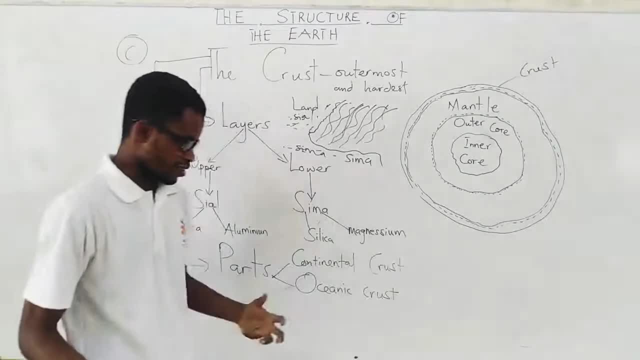 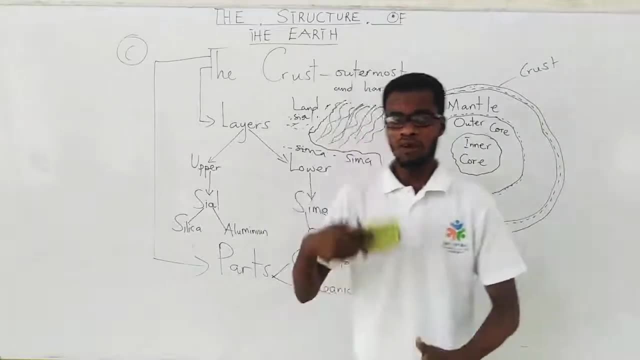 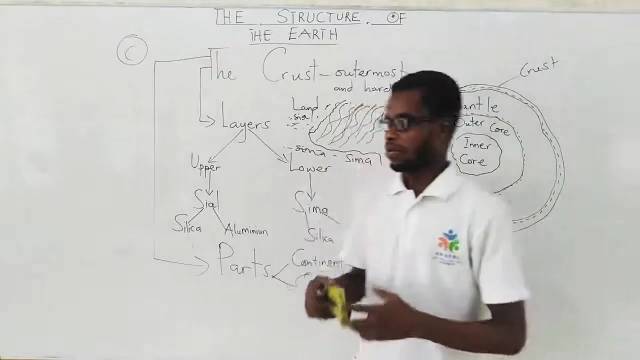 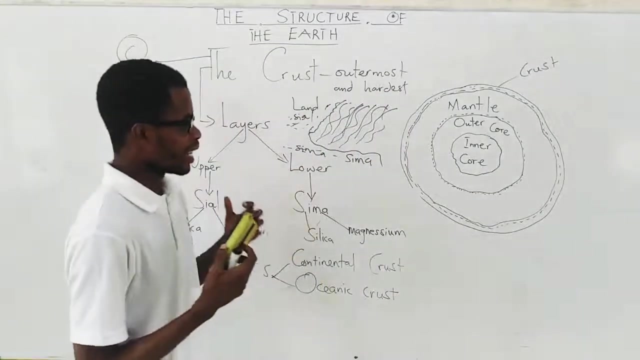 Then you have the part, The continental crust and the oceanic crust. All these substances and other elements are found within the layers of the earth And we keep on tapping them as resources to serve mankind. to serve mankind No matter how hidden they are in the earth. we try to bring them out since we need them for the earth. 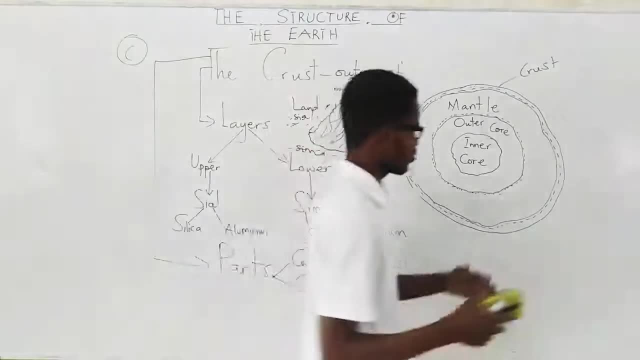 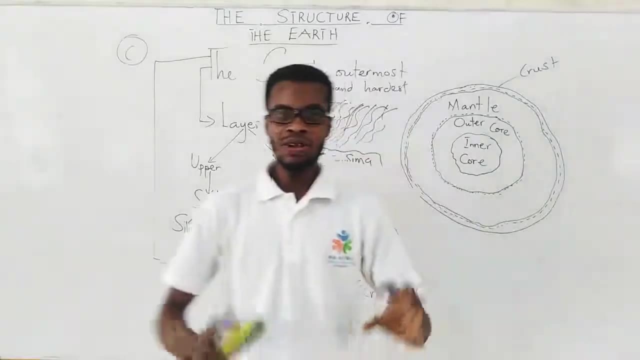 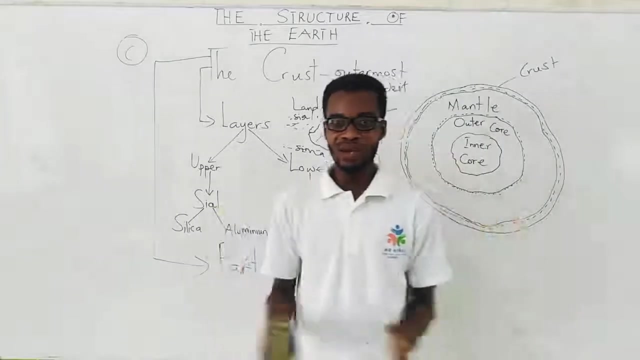 For the satisfaction of whatever useful thing that mankind needs or wants. All right, So this is a brief description of the structure of the earth, All right. So, dear Eleanor, I am sure you have learned a lot about the structure of the earth.